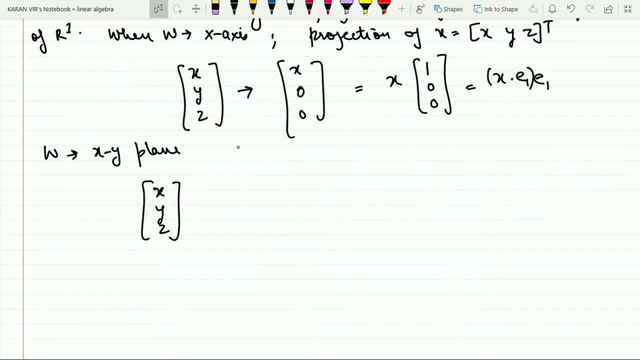 Similarly, if my w comes out to be x y plane, And what is the projection in this case? of x y z, So that is x y 0.. And in this case you can write it down: x into 1, 0, 0 plus y times 0, 1, 0,. 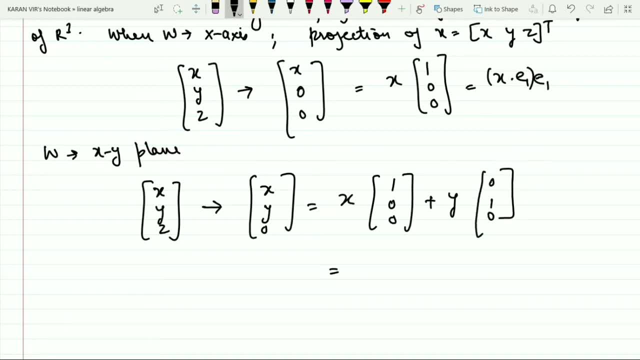 right. So now, furthermore, you can write it down like: x dot with e1 multiply with e1, plus x dot with e2 multiply with e2.. So that is the intuitive idea how we, you know, check the projection of this. Now let me formally define the orthogonal projection So as to make you think more. 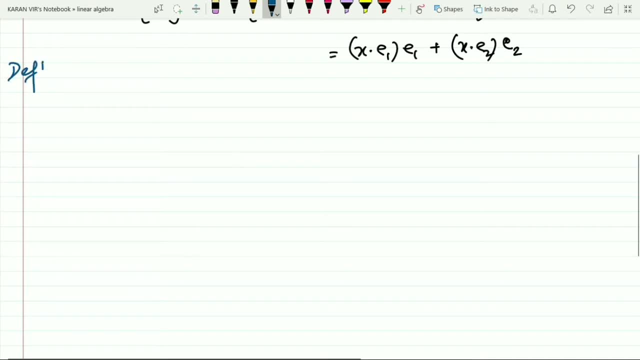 clear. So the formal definition for this: we will consider w to be any linear subspace, So w be a linear subspace of Rn, And then you will consider any vector that is coming from Rn. that is, let x come from Rn. So what is the orthogonal projection? That is what we are considering right. So if 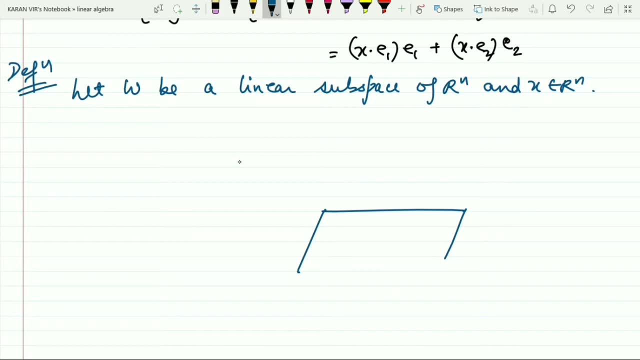 see, this is my, so let me draw it here. So if this is my, my subspace, I have called it as w. right Now, if this is any arbitrary vector x, fine with this. Now I want the orthogonal projection, So it means I have to draw vector. 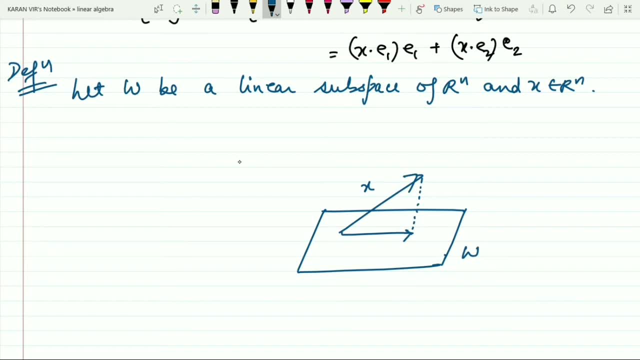 in this direction and this direction. Fine with this. So this is the projection, that is, if you see, from O to B, this will be the projection of OA, vector right, That is a, y. So so if, for this, now let me write it So- w be a linear subspace of Rn and x, 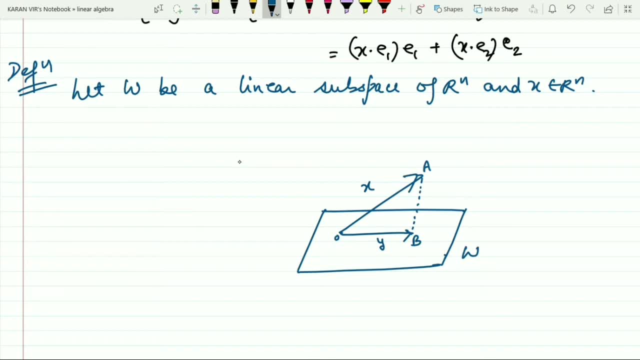 you have considered to be any vector in Rn, then a vector, a vector y, right. So this is a vector y, you can see in the figure in w. So a vector y in w, such that x minus y is perpendicular to w. So 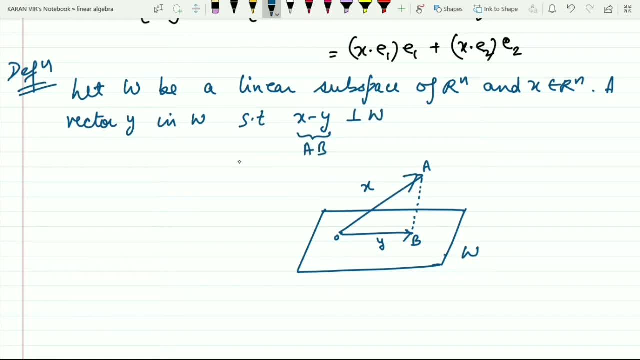 what is this? x minus y? This is nothing but AB. You can just visualize this, that this AB vector is nothing but normal to this subspace. Now even you can just check it out how I can write it down like x minus y. 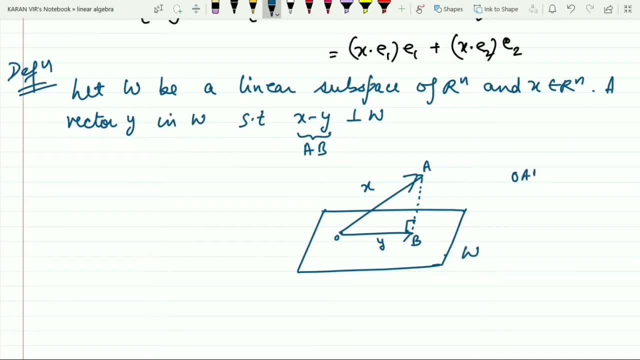 Because if you apply the triangles law in this OAB, triangles law right. So OB plus AB is equals to OA, right? So what is my AB? AB is nothing but OA minus OB, right? What is my OA? That is x. 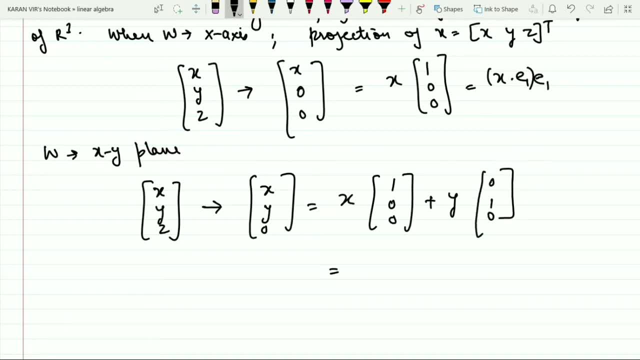 right. So now, furthermore, you can write it down like: x dot with e1 multiply with e1, plus x dot with e2 multiply with e2.. So that is the intuitive idea how we, you know, check the projection of this. Now let me formally define the orthogonal projection So as to make you think more. 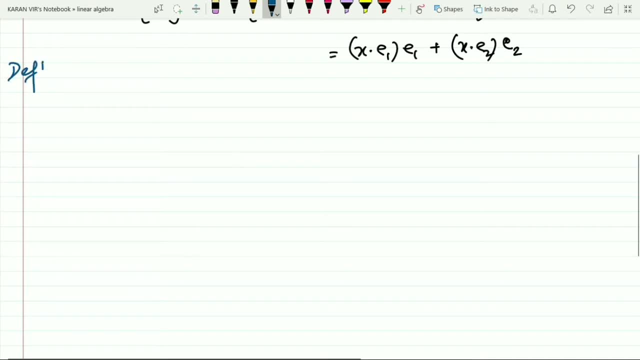 clear. So the formal definition for this: we will consider w to be any linear subspace, So w be a linear subspace of Rn, And then you will consider any vector that is coming from Rn. that is, let x come from Rn. So what is the orthogonal projection? That is what we are considering right. So if 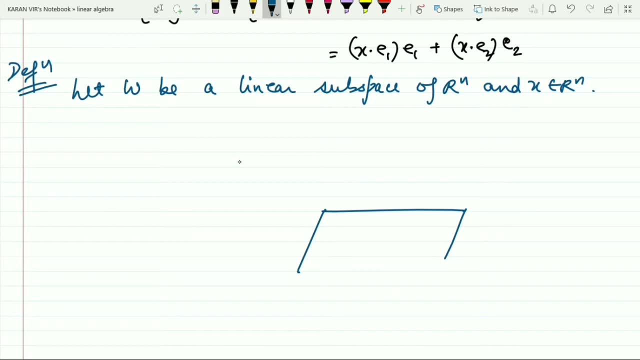 see, this is my, so let me draw it here. So if this is my, my subspace, I have called it as w. right Now, if this is any arbitrary vector x, fine with this. Now I want the orthogonal projection, So it means I have to draw vector. 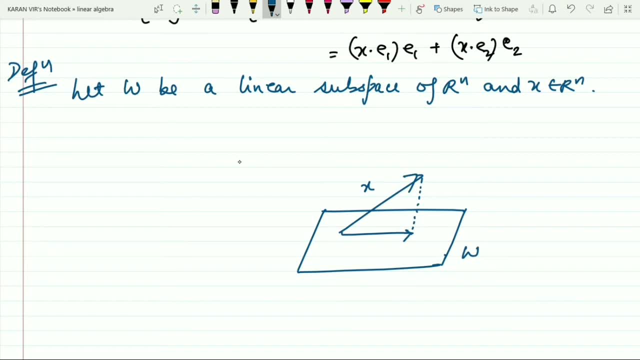 in this direction and this direction. Fine with this. So this is the projection, that is, if you see, from O to B, this will be the projection of OA, vector right, That is a, y. So so if, for this, now let me write it So- w be a linear subspace of Rn and x, 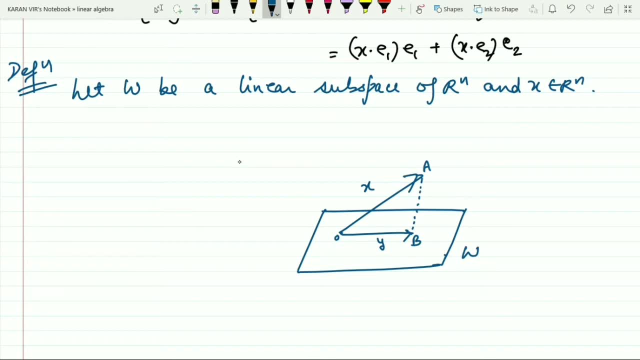 you have considered to be any vector in Rn, then a vector, a vector y, right. So this is a vector y. you can see in the figure in w. So a vector y in w, such that x minus y is perpendicular to w. 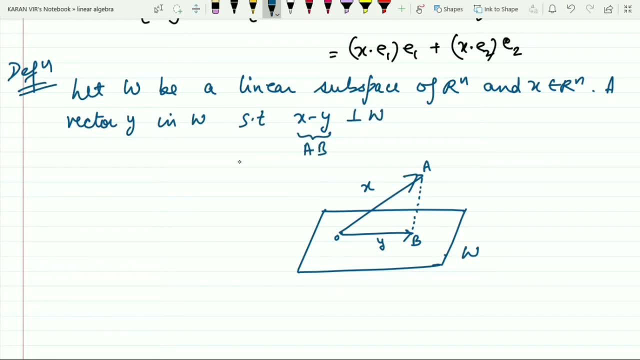 So what is this? x minus y? This is nothing but AB. You can just visualize this, that this AB vector is nothing but normal to this subspace. Now even you can just check it out how I can write it down like x minus y. 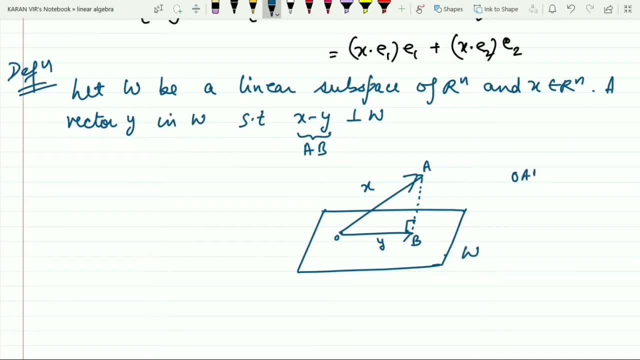 Because if you apply the triangles law in this OAB, triangles law right. So OB plus AB is equals to OA, right? So what is my AB? AB is nothing but OA minus OB, right? What is my OA? That is x. 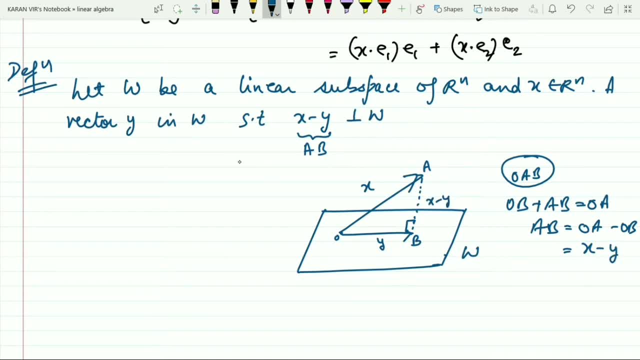 What is this Y? So AB comes out to be nothing but x minus y. So can I say this: x minus y is perpendicular to this subspace w, right? So if w is my linear subspace of Rn and x is any vector, 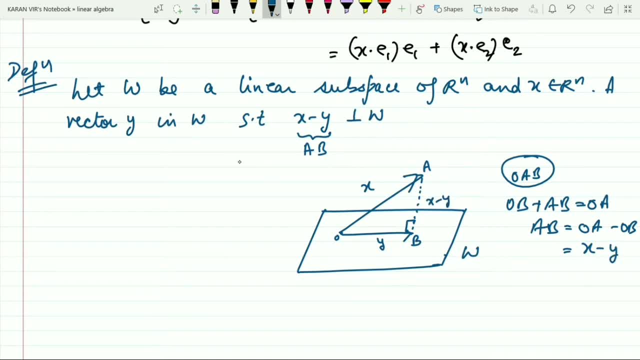 What is this Y? So AB comes out to be nothing but x minus y. So can I say this: x minus y is perpendicular to this subspace w, right? So if w is my linear subspace of Rn and x is any vector, 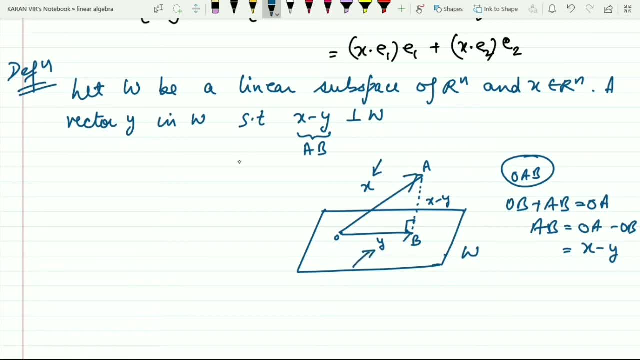 coming from Rn. so this vector y is called the projection right. So this is called the, this vector is called the orthogonal projection, So orthogonal projection of this vector x to the w, And when I will say this is a orthogonal projection. 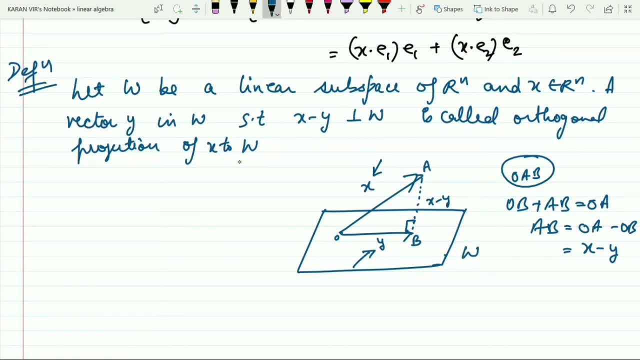 if x minus y, so that is such that x minus y is perpendicular to this subspace, right? So if my x minus y is perpendicular to this subspace w? so there is a notation which I will generally call. that is this: x minus y. this will go to, so I will say that x minus y. 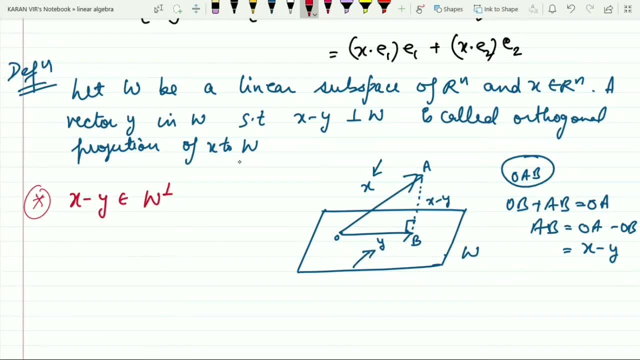 belongs to w perpendicular, that is, a perpendicular subspace, right? So so, final result: what is the result? What is the conclusion? Conclusion is: whenever my x minus y is perpendicular to w. So this is if, and only if, my x minus y belongs to w perpendicular. right Now let me consider. 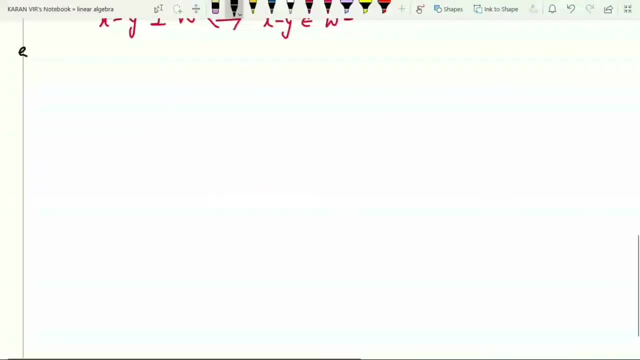 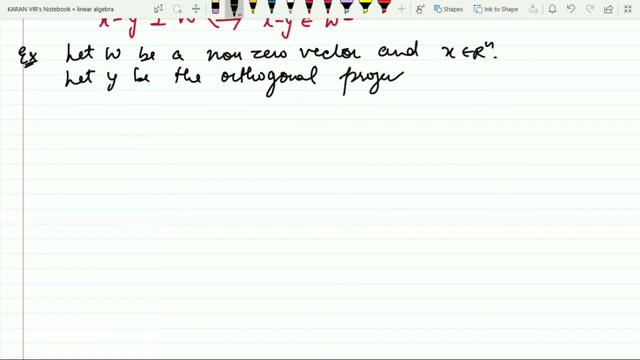 an example for this. So example: so let w be a non-zero vector and x is any vector coming from Rn right And let y be the orthogonal projection, orthogonal projection of x to the line that is spanned by w. So y is characterized by. so y will come from w right And x minus y. so see this, this x minus y. 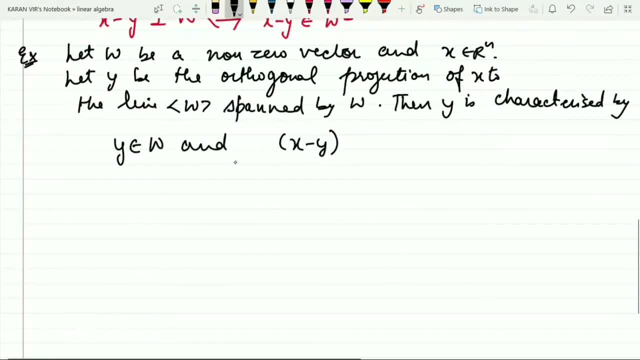 right. If you take the dot with w, w is any vector, so that will come out to be zero because it's perpendicular and right to this space. So whenever you take the dot product of this, this will automatically comes out to be zero. Now, since y belongs to the 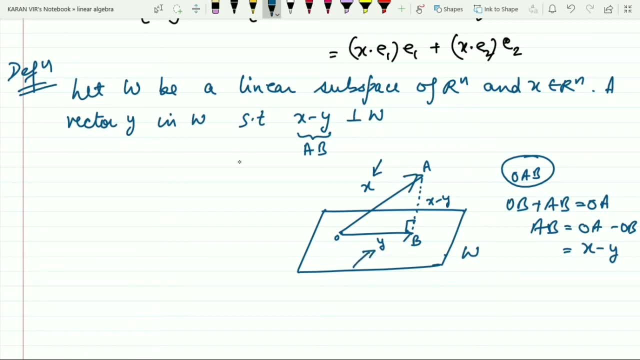 coming from Rn. so this vector y is called the projection right. So this is called the, this vector is called the orthogonal projection, So orthogonal projection of this vector x to the w, And when I will say this is a orthogonal projection. 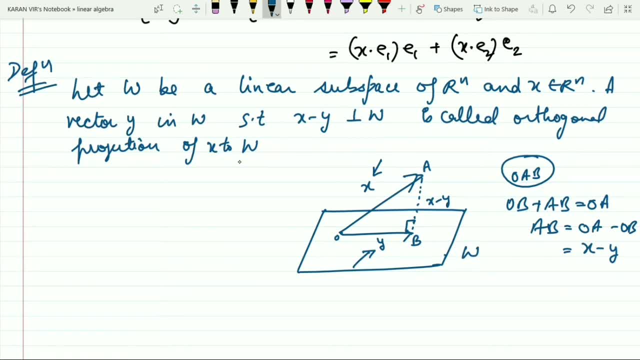 if x minus y, so that is such that x minus y is perpendicular to this subspace, right? So if my x minus y is perpendicular to this subspace w? so there is a notation Which I will generally call. that is this: x minus y. this will go to, so I will say that x minus y. 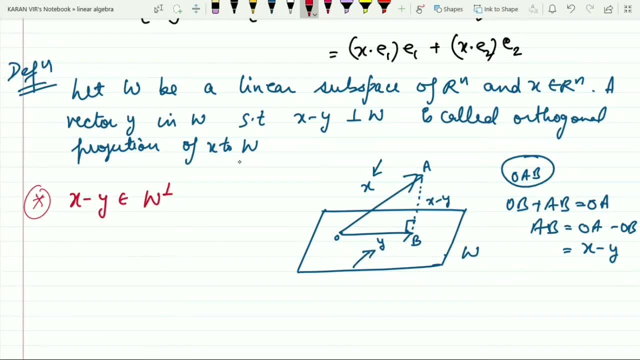 belongs to w perpendicular, that is, a perpendicular subspace, right? So so, final result: what is the result? What is the conclusion? Conclusion is: whenever my x minus y is perpendicular to w. So this is if, and only if, my x minus y belongs to w perpendicular. right Now let me consider. 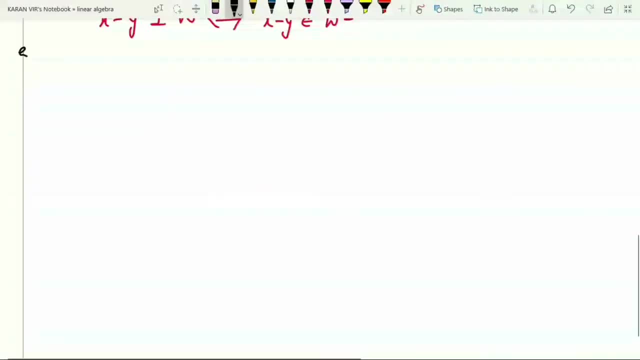 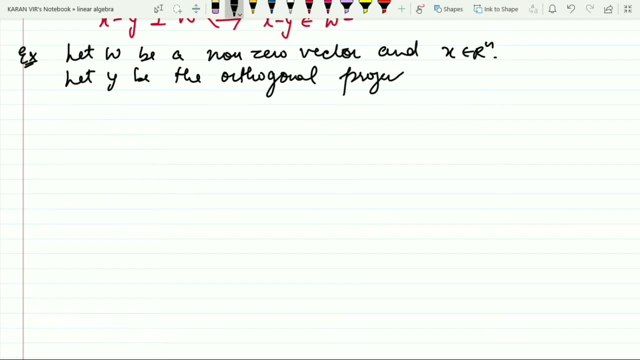 an example for this. So example: so let w be a non-zero vector and x is any vector coming from Rn right And let y be the orthogonal projection, orthogonal projection of x to the line that is spanned by w. So Y is characterized by. so y will come from w right And x minus y. so see this, this x minus y. 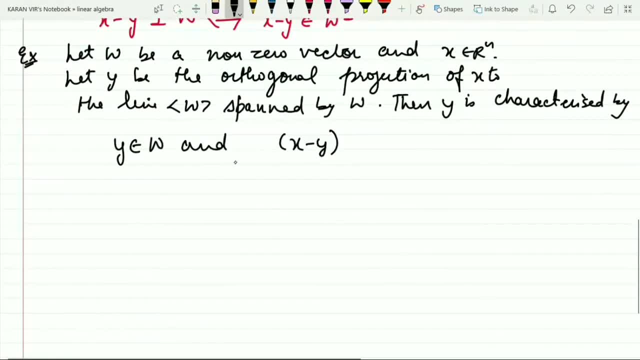 right. If you take the dot with w, w is any vector, so that will come out to be zero because it's perpendicular and right to this space. So whenever you take the dot product of this, this will automatically comes out to be zero. Now, since y belongs to the 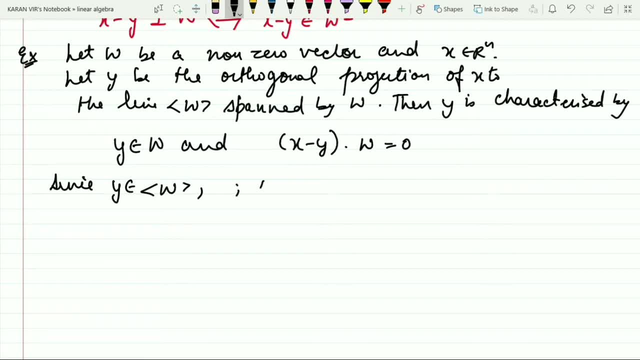 n of w, right. so can i say: y is some r times, w for some scalar r for some scalar r, right of course, coming from field, and the field is r. i have considered here, right. so see this. so what is my zero? zero is nothing but x minus y, dot with w. from this one equation, right now, just separate. 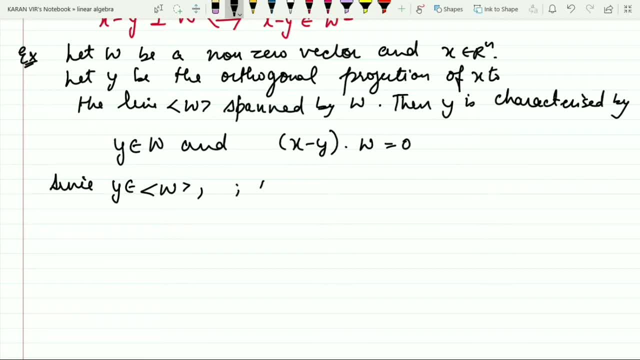 of w, right. So can I say: y is some R times, w for some scalar R for some scalar R, right, Of course, coming from field, and the field is R. I have considered here, right. So see this. So what is my zero? Zero is nothing but x minus y, dot with w. from this one equation. 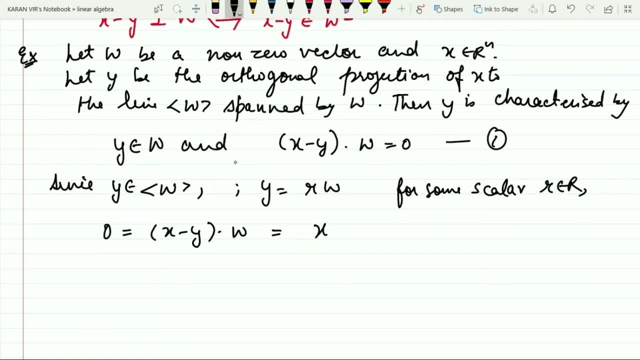 right Now. just separate these terms. So this will be x dot w right, Minus y dot w. and what is the value of y? That is R times w. just substitute the value here. I think up to this. the steps are clear. So this is x. so this is x dot w minus R times w dot with w. 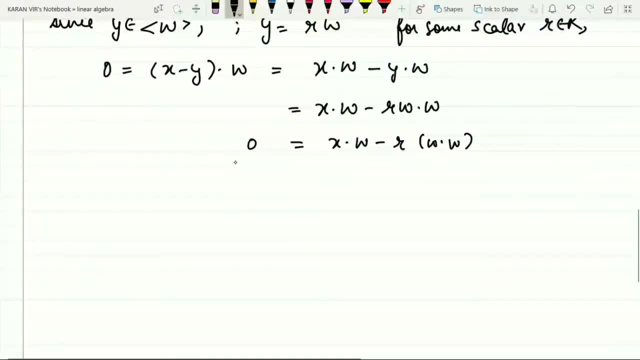 right Which yields that. so this is equals to zero. So can I say, can I say that this R is equals to. so just bring the terms on one side: R into w, dot with w is equals to x dot w. And what? 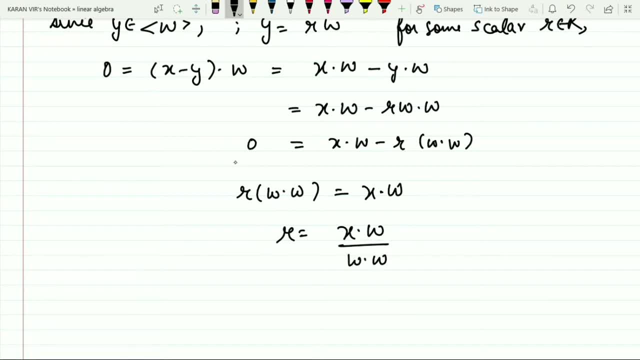 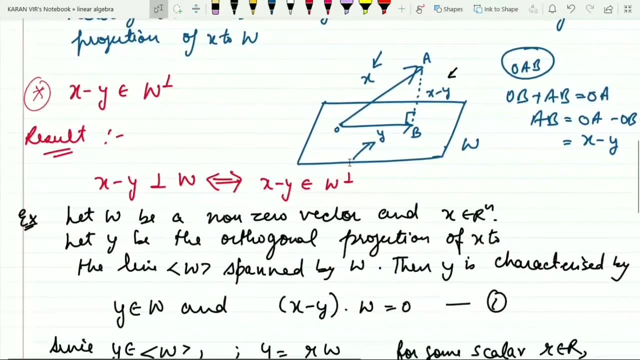 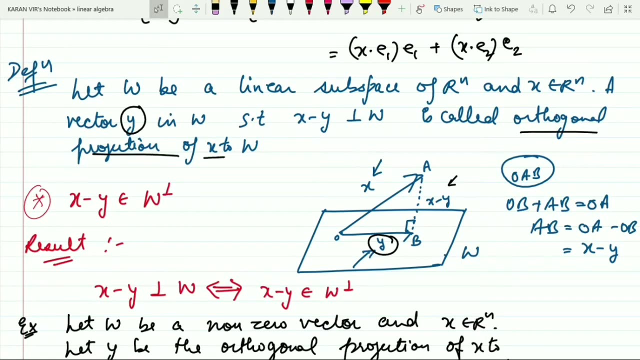 this value be is w dot w. Now, I don't know how to figure that. That is my common knowledge. We are only going to develop that value later. So what I want to do here we're going to see an R and we're going to substitute what I can get with R over. 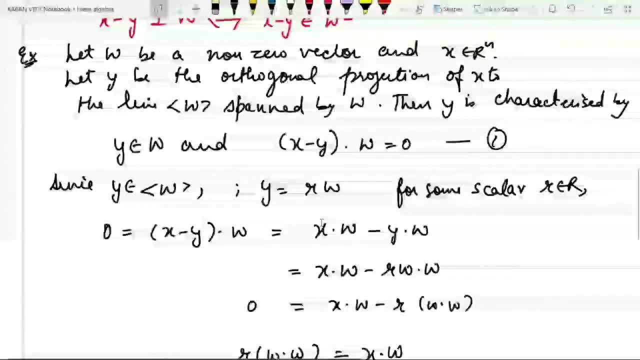 n with w. So, based on this expression, go back And we're essentially identifying that we can understand what I have to calculate with our function, This, it, and we have to look at our subject. So these table in this desses, which are indicated by this square piece, We're sealed by 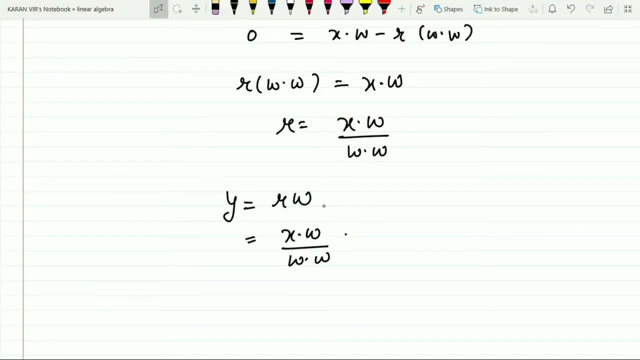 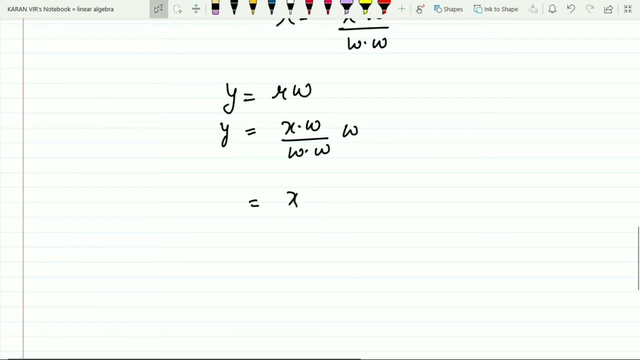 this: you divide by flying terms: X dot w minus R dot w. What about self square? 3 x dot w. rx dot w divide by w dot w multiply with w. So this is the value of r right and already I know that what is my w dot with w? that is nothing but norm of w square right multiply with w. 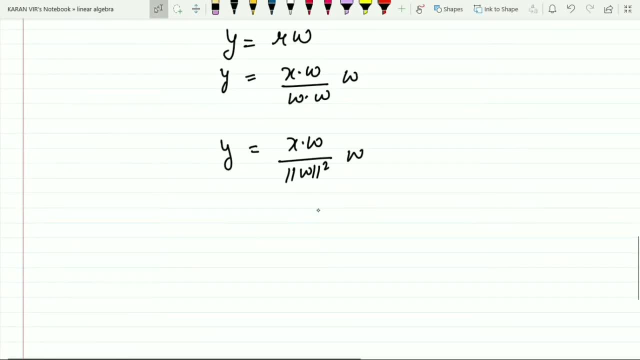 So that is the value of y. Now, conversely, if I say that the vector is given by the formula, So the vector y, given by above formula, certainly satisfies that y belongs to w, and x minus y dot with w is 0 right, So which gives rise to: 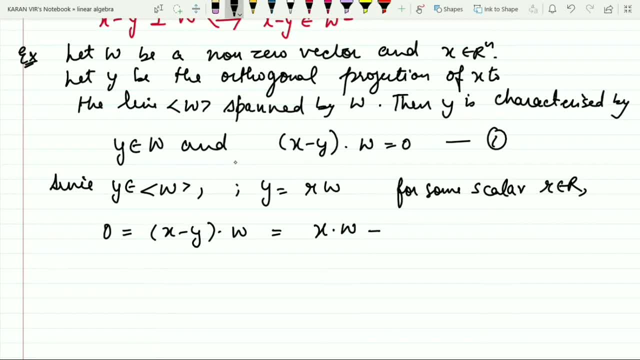 these terms. so this will be x dot w right minus y dot w. and what is the value of y? that is r times w. just substitute the value here. i think up to this. the steps are clear. so this is x. so this is x dot w minus r times w dot with w right, which yields that. so this is equals to zero. so can i? 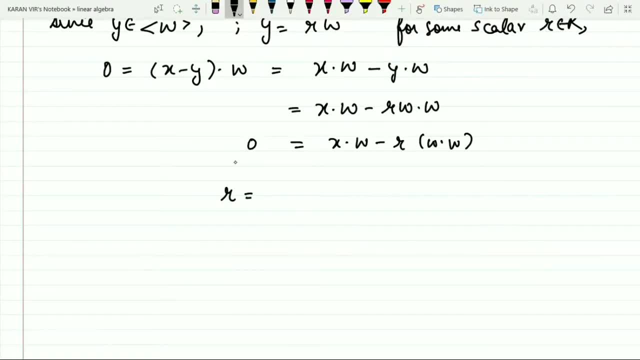 say. can i say that this r is equals to? so just bring the terms on one side, r into w dot with w is equals to x dot w. and what is the value of r? so this is x dot w divide by w dot with w. fine with this. so that is the value of r. and what were we interested? we were interested to calculate. 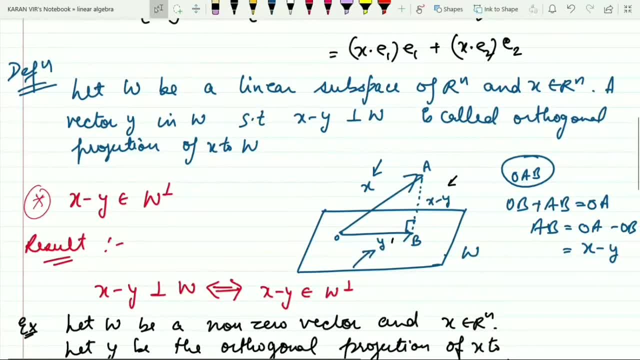 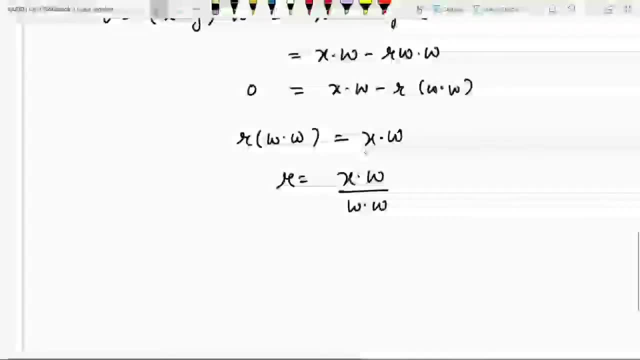 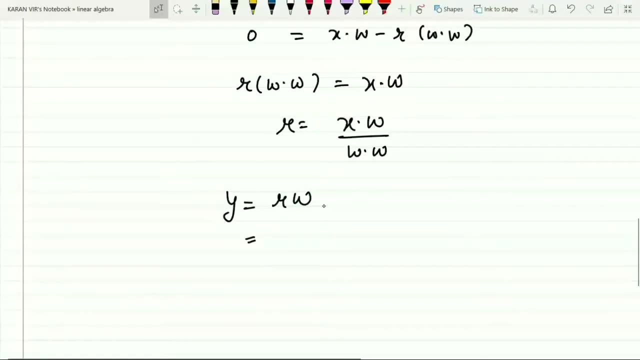 the value of y. why? because why we were interested to calculate the value of y, because the y is the orthogonal projection of x to this subspace and we want to know the value of y. so what was my y? we have considered the y to be right r times w. so just substitute it here: r times w. what is the? 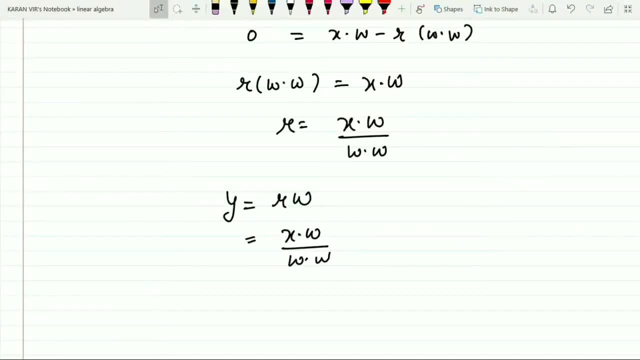 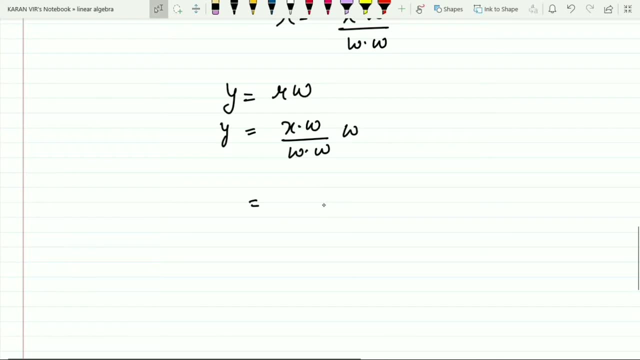 value of r x dot w divide by w dot w multiply with w. so this is the value of r right, and already i know that what is my w dot with w? that is nothing but norm of w square right multiply with w. so that is the value of y. now, conversely, conversely, if i say that the 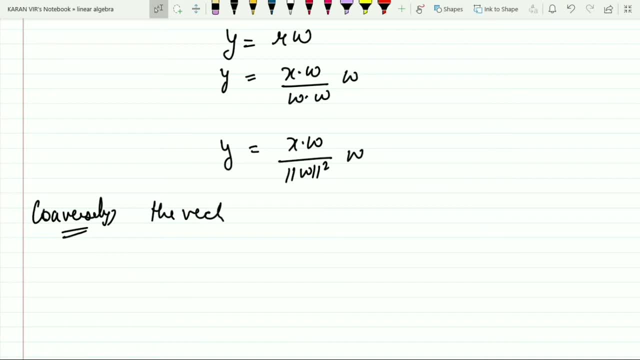 vector is given by the formula. So the vector y given by above formula certainly satisfies that y belongs to w, and x minus y dot with w is 0, right, So which gives y rise to orthogonal projection. orthogonal projection, right. 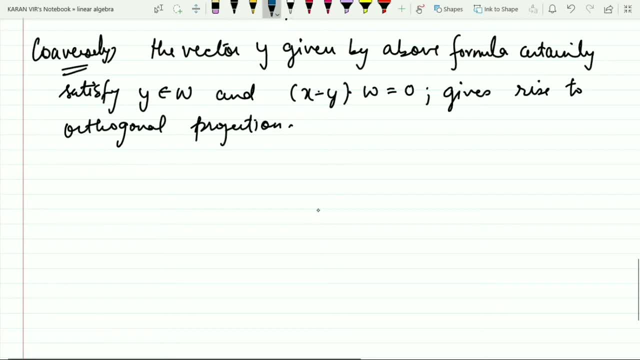 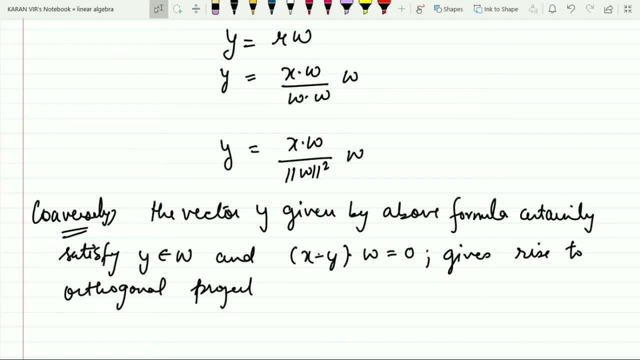 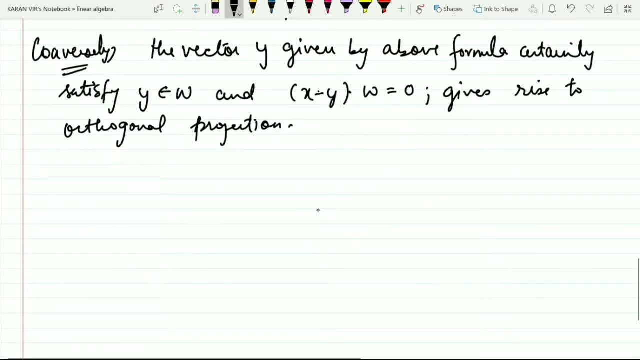 y dot ororthogonal projection. Now let me consider an example for this. So, for example, so if w is nothing but my 1, 1, 1 right, 1, 1, 1 right and x is any arbitrary vector that is? 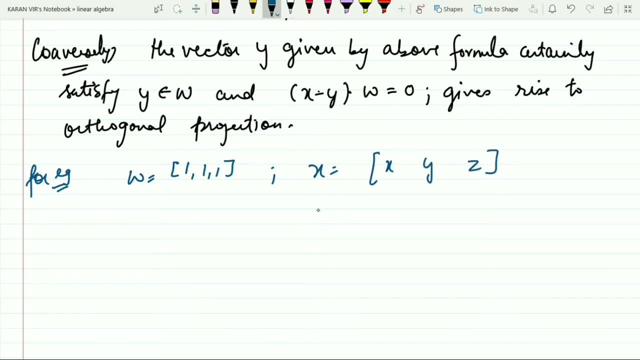 x, y and z right, and we want to calculate the projection of x, right. So that is nothing but 1, 1, 1.. So that is nothing but my 1 1, 1 right and x is any arbitrary vector, that is. 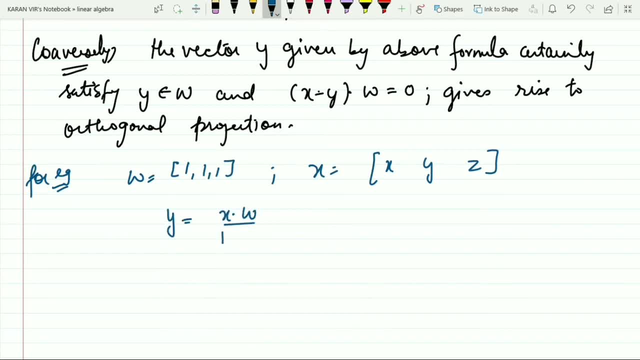 at y is equals to write x dot, w divide by w dot, w multiply with w. So just take the dot product of x and w. So this comes out to be x plus y plus z. and what is the w dot with w? that is 3, and what? 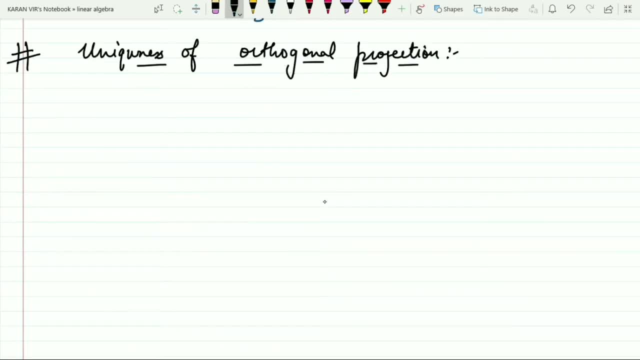 is the vector w, that is 1, 1, 1.. So now we discuss the uniqueness of orthogonal projection. that is, I want to prove that the orthogonal projection is always unique. So the theorem dealing with this is. so let me write the theorem. So if w is a linear subspace, w be a linear subspace. 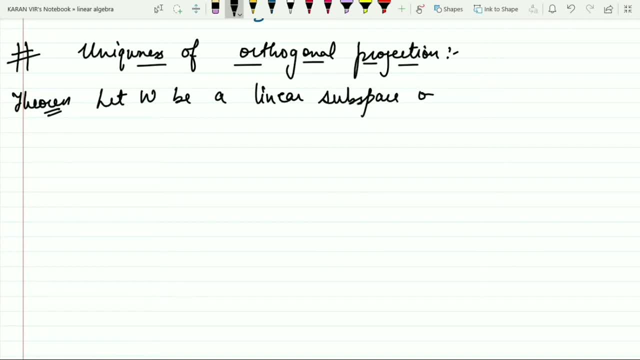 of Rn, and again you will consider any vector x coming from Rn. right? then the orthogonal projection. then the orthogonal projection, right, that is, of x to the w, is unique. that is what we are interested to prove, Right? So let me directly go to the proof, right? So for this, let y prime and y double prime. 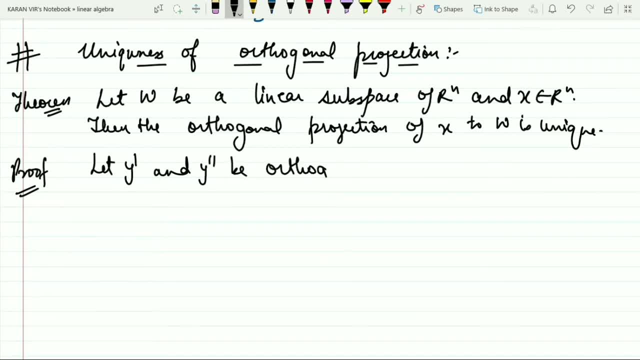 be the orthogonal projections, be the. So I will be considering two distinct orthogonal projections and finally, I have to prove that both of them are equal right. So let they be the orthogonal projections of x to the subspace, that is y, right Now what we are interested to prove. 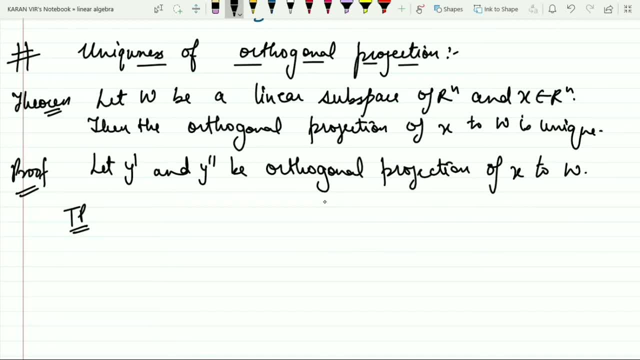 So we are what we want to prove: that y prime is nothing but y double prime, If we show this. So finally, we can say that the orthogonal projection is unique. for this let me consider. So let me set: z prime equals to x minus y. to calculate the projection of x, y and z. So we want to calculate the projection of x, y and z right And we want to calculate the projection of x, y and z right, And we want to. 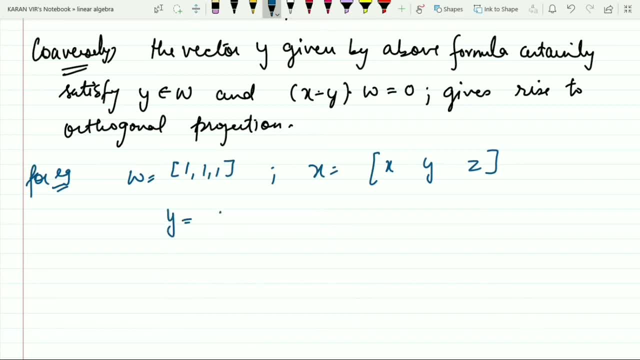 write x dot w divided by w dot w multiplied with w. So just take the dot product of x and w. So this comes out to be x plus y plus z. And what is the w dot with w? That is 3.. And what is? 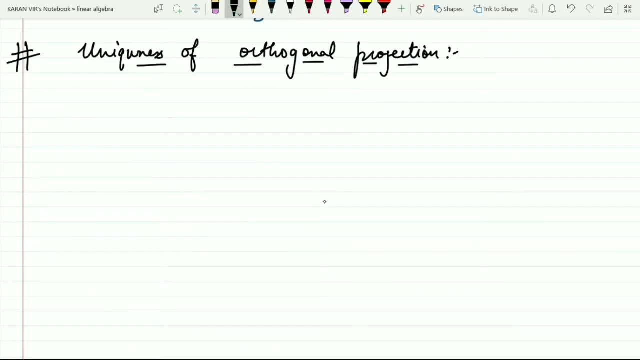 the vector w, That is 1,, 1, 1.. So now we discuss the uniqueness of orthogonal projection. That is, I want to prove that the orthogonal projection is always unique. So the theorem dealing with this is so let me write the theorem. So if w is a linear subspace, 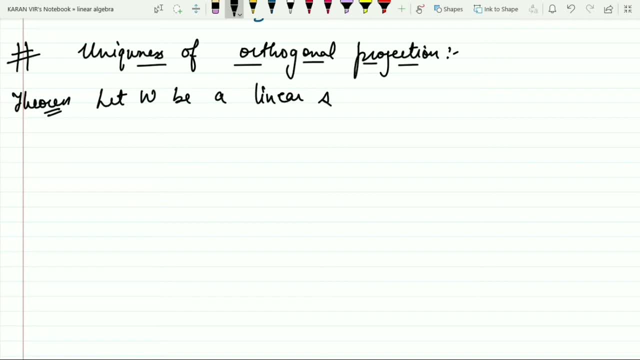 w be a linear subspace of Rn. And again, you will consider any vector x coming from Rn right, Then the orthogonal projection, then the orthogonal projection, right that is, of x to the w is unique. That is what we are interested to prove right. So let me 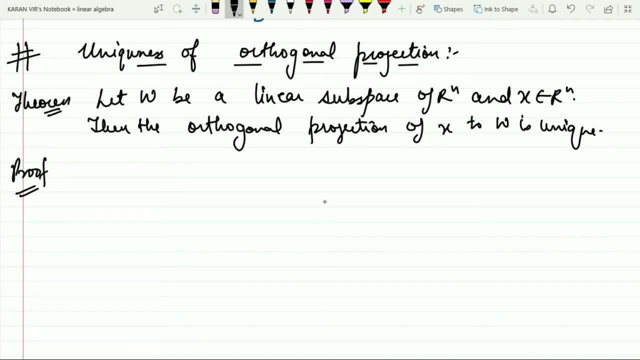 directly go to the proof. So for this, let y prime and y double prime be the orthogonal projections. So I will be considering two distinct orthogonal projections And finally I have to prove that both of them are equal right. So let they be the orthogonal projections of x to that subspace, that is y. 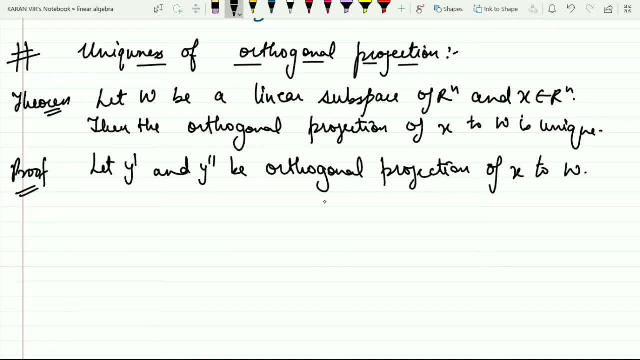 right Now what we are interested to prove. So we are what we want to prove: that y prime is nothing but y double prime If we show this. so finally, we can say that the orthogonal projection is unique. For this, let me consider: 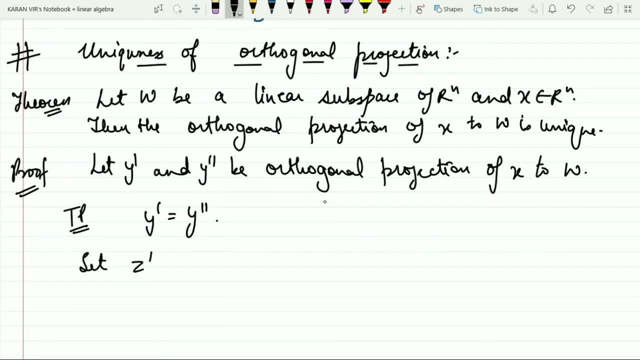 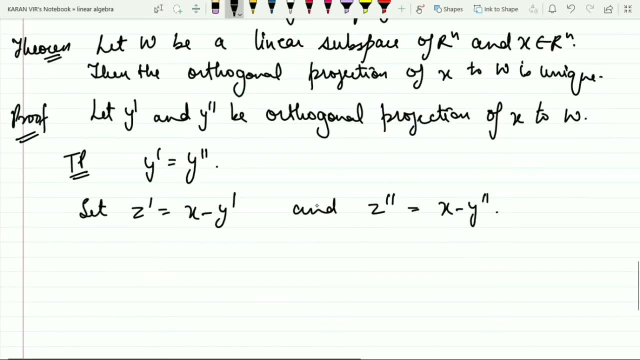 so let me set: z prime equals to x minus y prime, and z double prime equals to x minus y double prime. So, students, you can easily see this. So this is, if this was my subspace, as I would described above, and this is my vector x right, So the projection of this vector right. So 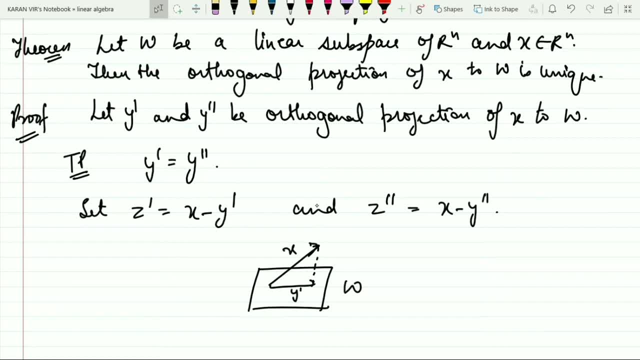 that is y prime in first case and the y prime in the another case. So, and what is this? This is nothing but my x minus y prime. So in the first case you have considered as z prime and in the other case you will be considering as a. 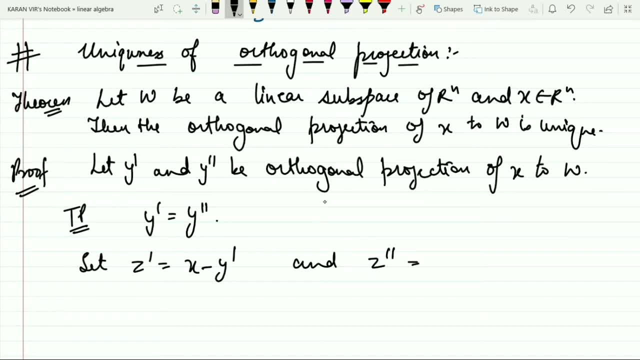 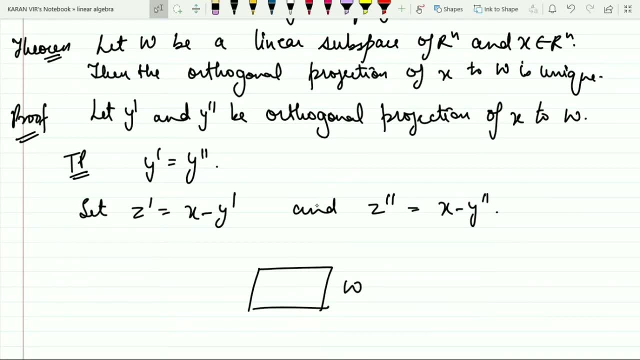 prime and z double prime equals to x minus y double prime. So, students, you can easily see this. So this is, if this is was my subspace, as I would described above, and this is my vector x right, So the projection of this vector right. So that is y. 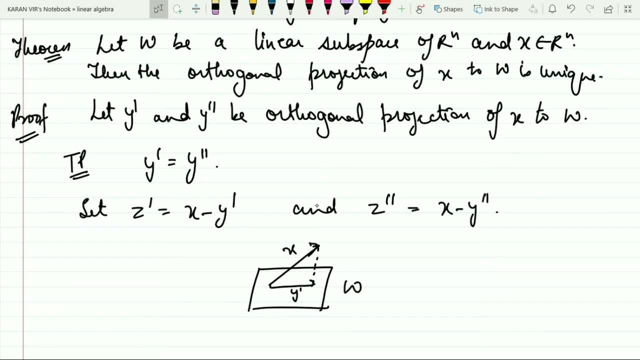 So this is my vector x right, So the projection of this vector right. So that is y prime in first case and the y prime in the another case. So, and what is this? This is nothing but my x minus y prime. So in the first case you have considered as z prime. 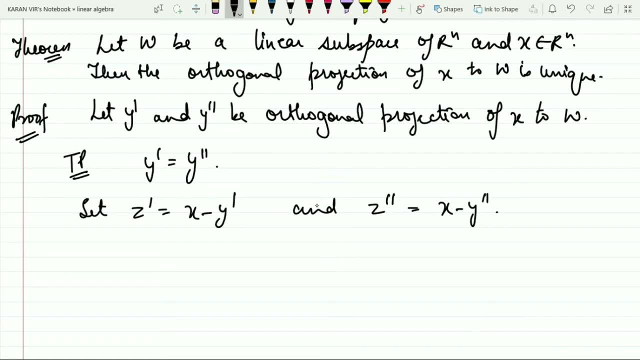 and in the other case you will be considering as a z double prime. So that is how I have set this: z prime and z double prime. So I hope this thing is clear to you now. So this implies x is equals to z prime plus y prime and x is equals to z double prime plus y double. 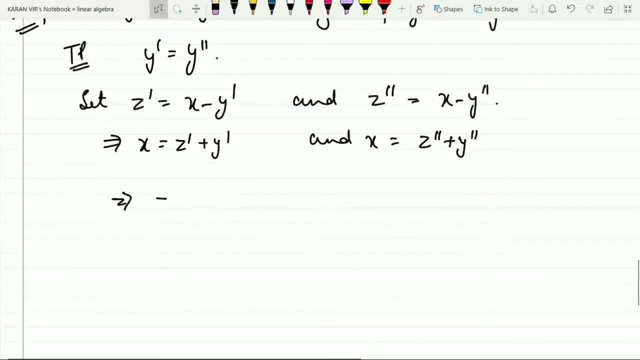 prime. So x is equals to both of these things. So this implies z prime plus y prime has to be equal to z double prime plus y double prime. or can I say: y prime minus y double prime is equals to z double prime minus z prime. right, And now you should observe one. 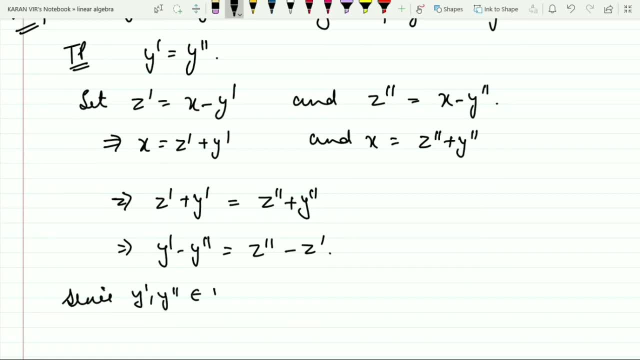 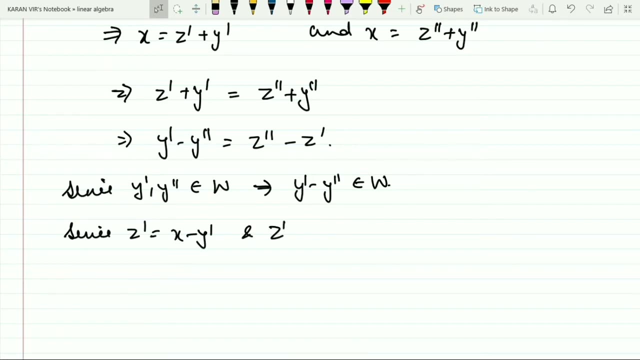 thing. So since y prime and y double prime, they were coming from w right and w is a subspace, so this implies y prime minus y double prime will also come from w right. And since, and since what was my z prime? z prime was x minus y prime right and z double prime was x minus y double. 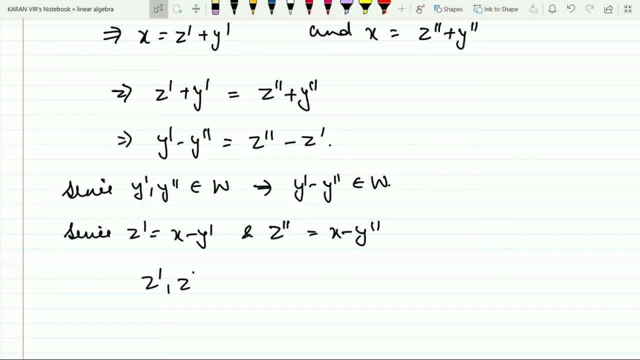 prime right, And both of these, z prime and z double prime, they belongs to w perpendicular subspace right, So again w perp, and w perp we have already proved that this is a subspace. So this implies z double prime minus z prime must belongs to w perpendicular, Fine with. 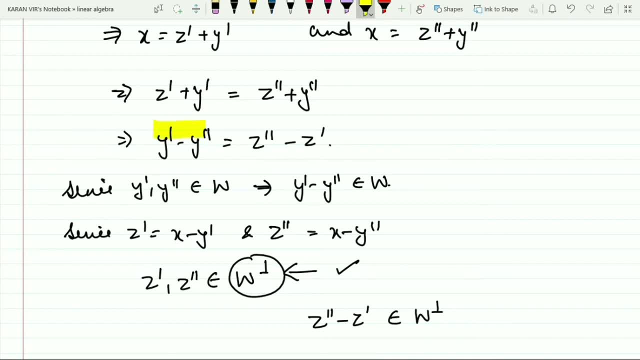 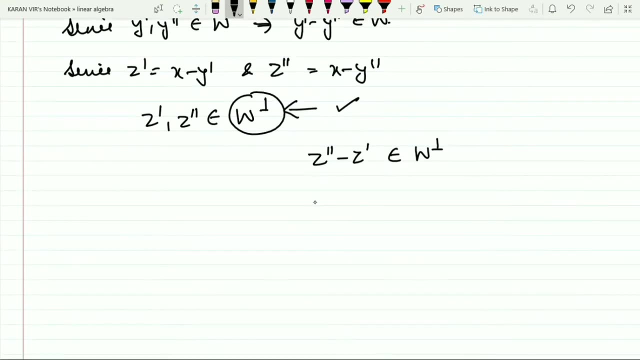 this. Now you should observe that here is the equality. Now one side, the one side belongs to w And the other side belongs to w perp. So this implies that that so the above equality, above equality will only hold, will only hold right when w intersection, w perp is nothing. 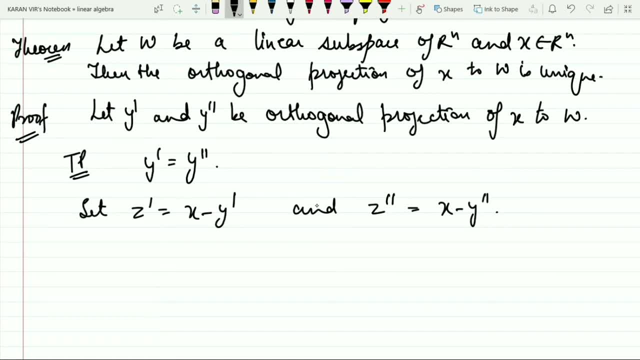 z double prime. So that is how I have set this: z prime and z double prime. So I hope this thing is clear to you now. So this implies x is equals to z prime plus y prime, and x is equals to z double prime plus y double prime. So x is equals to both of these things. 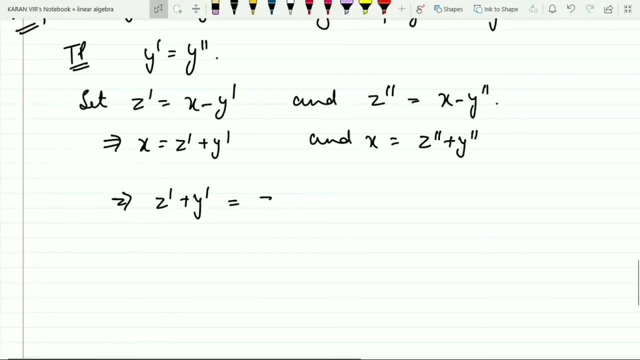 So this implies z prime plus y prime has to be equal to z double prime plus y double prime. So I can say y prime minus y double prime is equals to z double prime minus z prime. right, And now you should observe one thing. So since y prime and y double prime, they were coming. 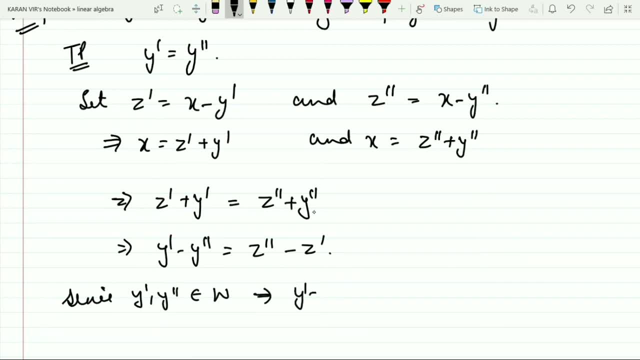 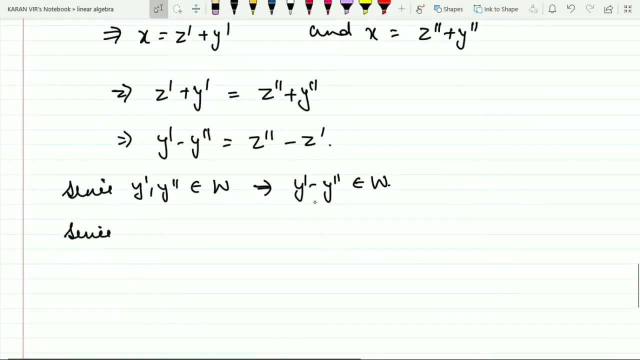 from w right And w is a subspace, So this implies y prime minus y. double prime will also come from w right And since, and since what was my z prime, z prime was x minus y prime right and z double prime was x minus y double prime right and both of these z prime. 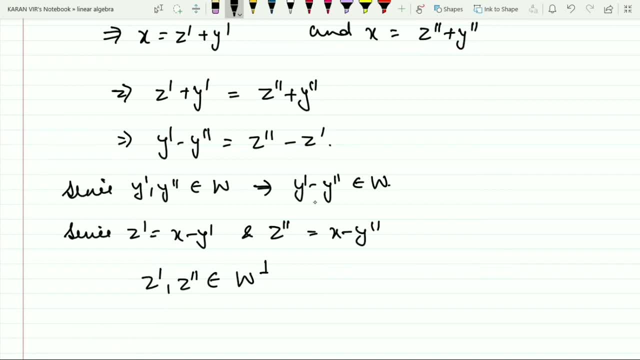 and z double prime. they belongs to w perpendicular subspace, right? so again, w perp and w perp. we have already proved that this is a subspace. so this implies z double prime minus z prime must belongs to w perpendicular. fine with this now. now you should observe that here is the equality, now one. 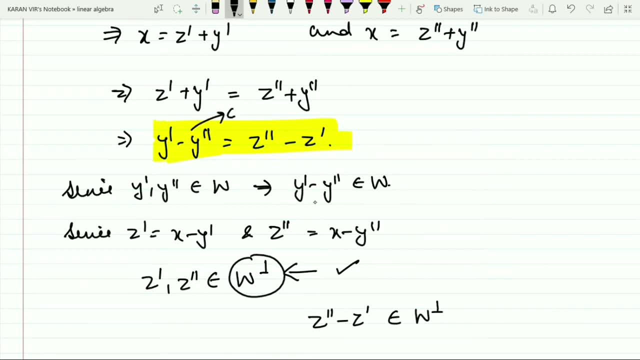 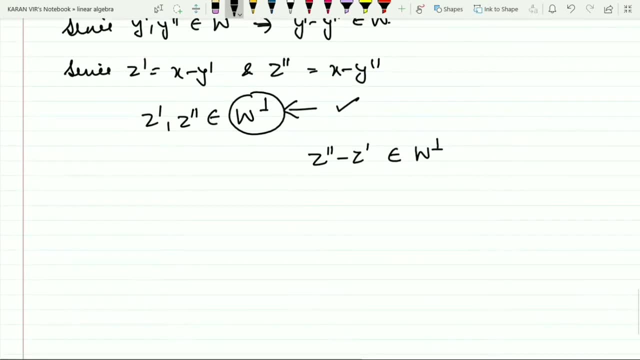 side. the one side belongs to w and the other side belongs to w perp. so this implies that that so the above equality, above equality will only hold, will only hold right when w intersection w perp is nothing but zero and if w intersection 0.. 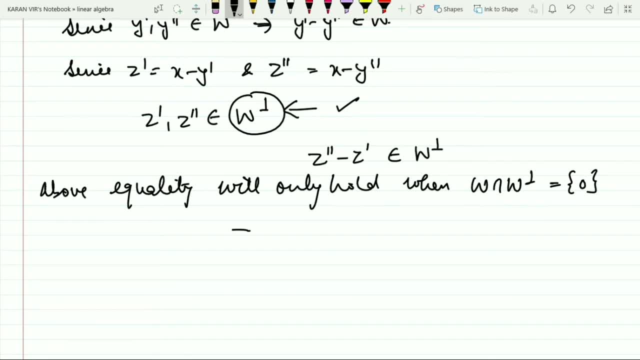 w perp is 0, right? So what does this implies? This implies that y, so they have to be equal to 0. So y prime equals to y double prime and z prime equals to z double prime, and hence uniqueness is proved. So let me repeat it once again for you. So since here it was equality, 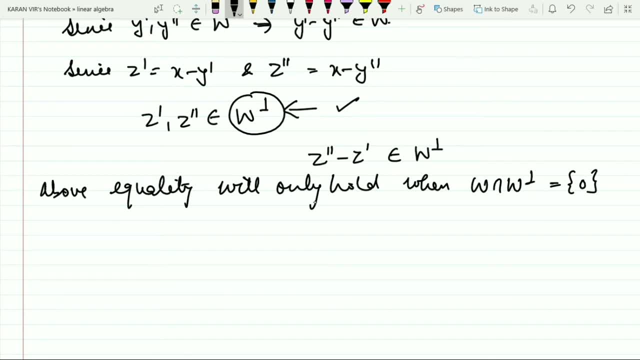 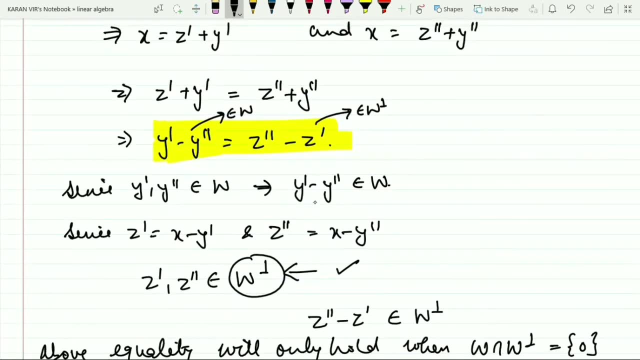 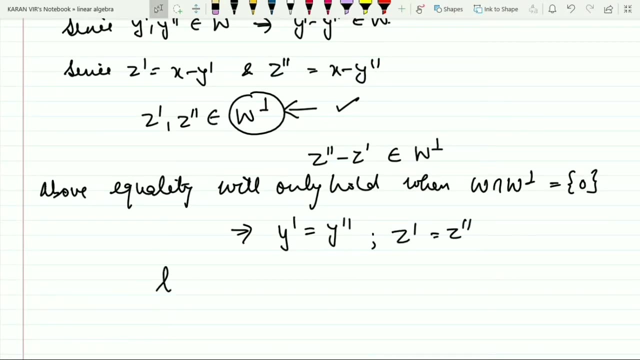 but zero. And if w intersection, w perp is zero, right. So what does this implies? This implies: this implies that y, so they have to be equal to zero, So y prime equals to y double prime and z prime equals to z double prime, and hence uniqueness is proved. 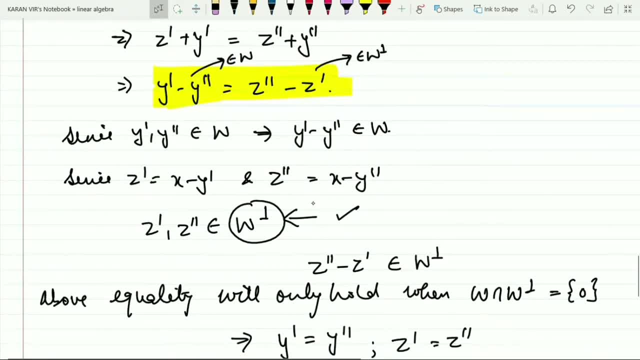 Let me repeat it once again for you: So since there it was equality, one side was belonging to w, the other side was belonging to w perp. So they have nothing in common except zero right. So that is, that is the common between the two subspaces. 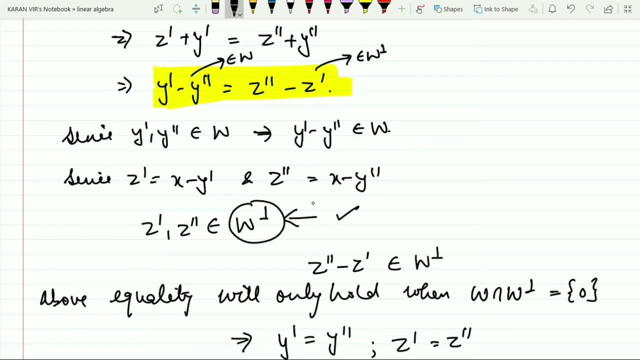 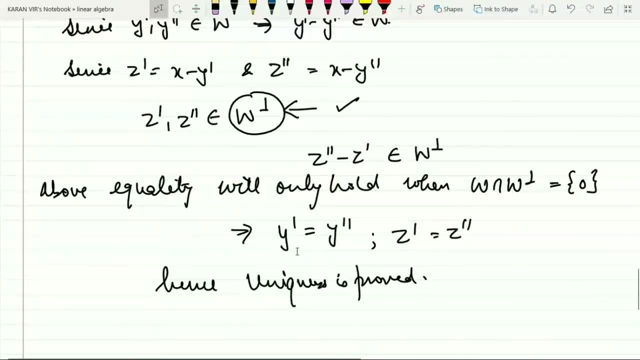 So finally, y prime minus y double prime and z double prime minus z prime, they have to be equal to zero. And if my y primes comes out to be equal to y double prime, and that is how we have, you know, proved the uniqueness. So the next topic is finding the orthogonal. 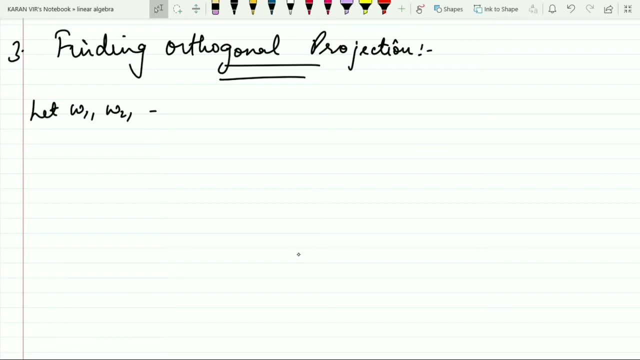 projections. for this let me consider w1, w2 up till wk. right, They forms an orthogonal basis. Then we will have y prime minus y double prime and z double prime minus z prime. they have the orthogonal projection of the vector x right to w is given by. already we have described the above formula right and 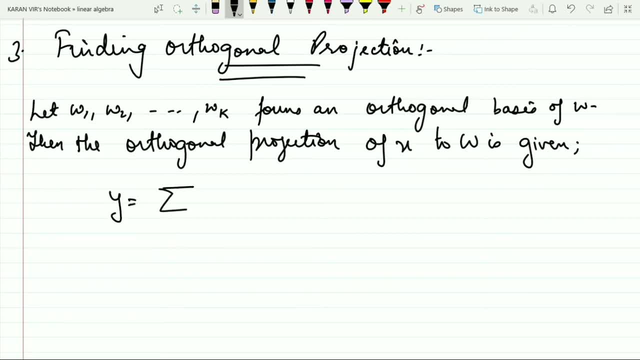 now we can write the formula in the summation form. so y comes out to be equal to summation. i, running from 1 to k, x dot with w, right wi, right wi dot with wi. multiply with wi, and you can furthermore write it down: that is the summation. i, running from 1 to k, x dot, wi, and what is wi dot? 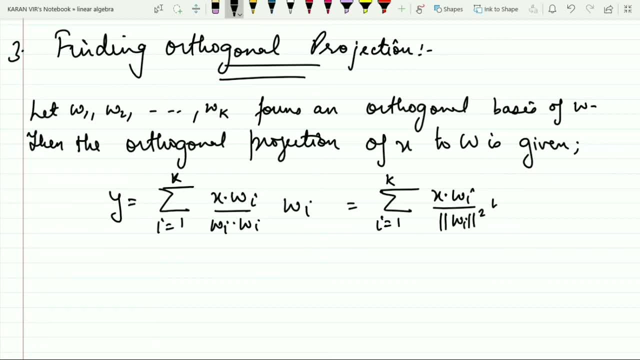 with wi. that is norm of wi: square multiply with wi. so that is the formula, right? so since y is a linear combination, linear, so you can see y is summation times wi, right? so something times w1 plus something times w2 plus something times w3, up till so on to something same wk. so can i? 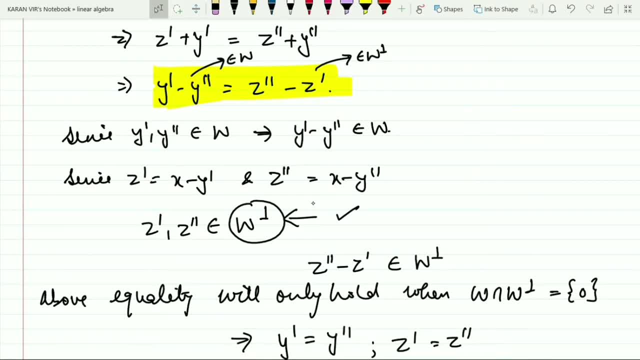 one side was belonging to w, the other side was belonging to w perp. So they have nothing in common except 0, right? So that is the common between the two subspaces. So finally, y prime minus y double prime and z double prime minus z prime, they have to be equal to 0. And if my y 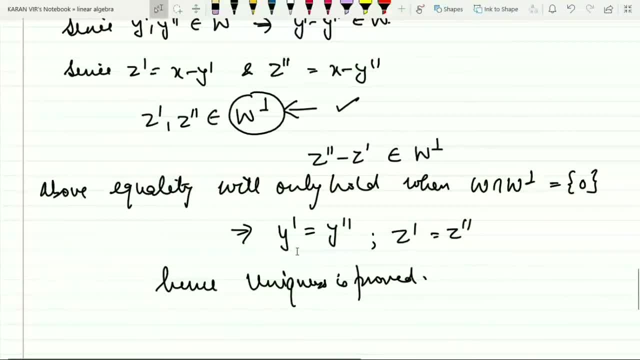 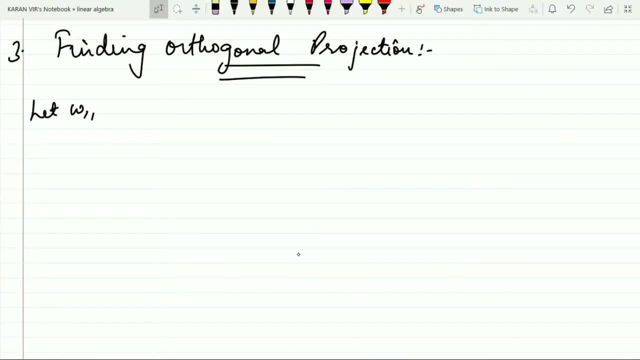 primes comes out to be equal to y double prime, and that is how we have, you know, proved the uniqueness. So the next topic is finding the orthogonal projections. For this. let me consider w1, w2, up till wk. right, They forms an orthogonal basis. 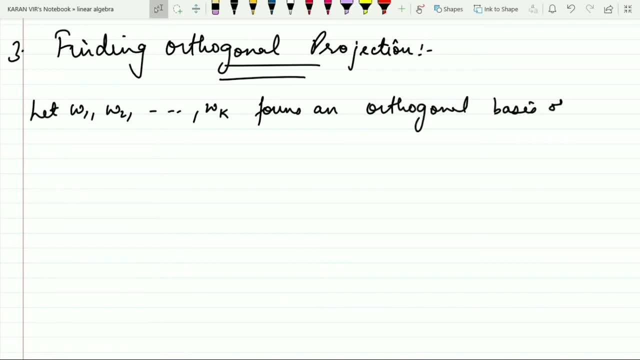 Then the orthogonal projection of the vector x right to w is given by. already we have described the above formula right, And now we can write the formula in the summation form. So y comes out to be equal to summation. 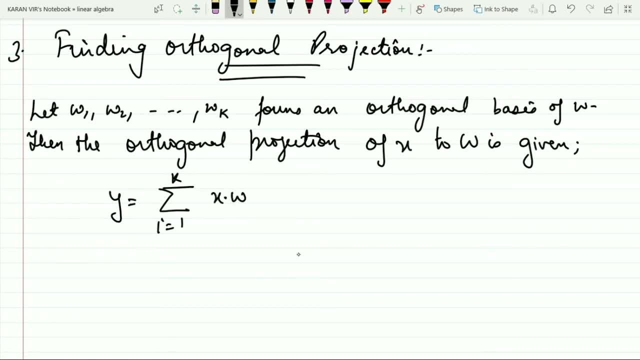 i running from 1 to k, x dot with w right, wi right. So y prime is equal to y double prime multiplied wi dot with wi. multiply with wi And you can furthermore write it down. That is the summation. i, running from 1 to k, x dot wi And what is wi dot with wi? That is norm of wi square. 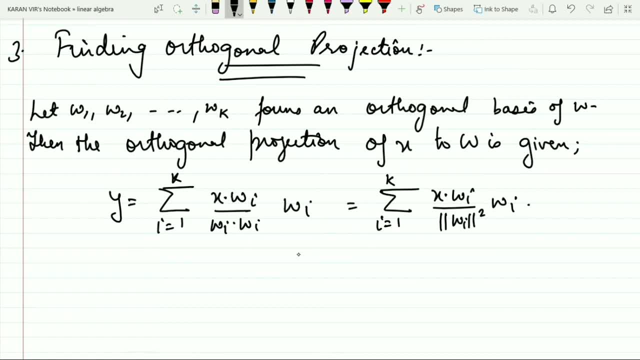 multiply with wi. So that is the formula, right. So since y is a linear combination, linear, so you can see y is summation times wi, right? So something times w1 plus something times w2 plus something times w3 plus something times w4 plus something times w5 plus something times w6 plus. 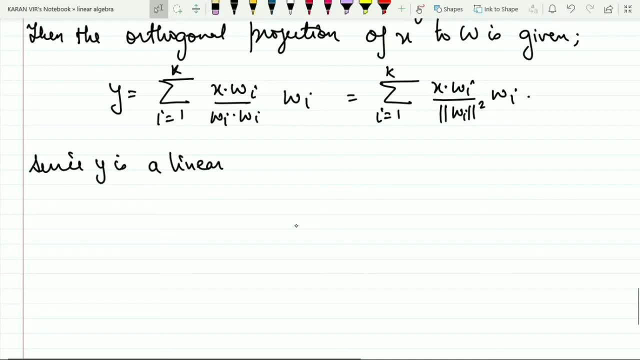 something is w3, up to something side wk. So can I say y is a linear combination, linear combination of w1, w2 up till so on to wk, right. So it belongs to w, right. So now, if you calculate x minus y, dot with wj, so what does it comes out to be? So 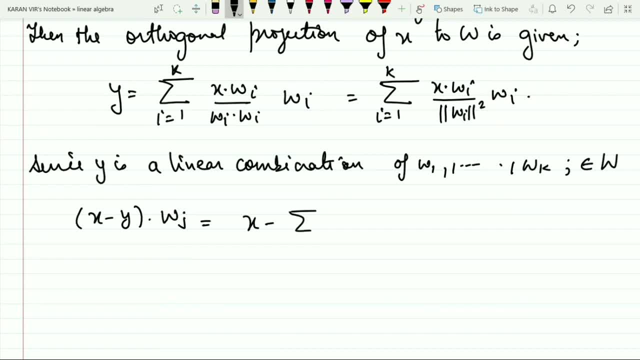 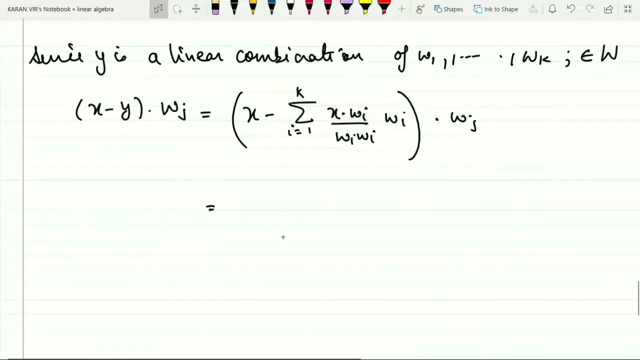 it comes out to be x minus. what is the value of y? y is summation i running from 1 to k right: x dot wi, divide by wi, dot with wi, multiply with wi and whole dot with wj. now just club the terms. so this is x? dot wj minus. summation i running from 1 to k: x dot wi. 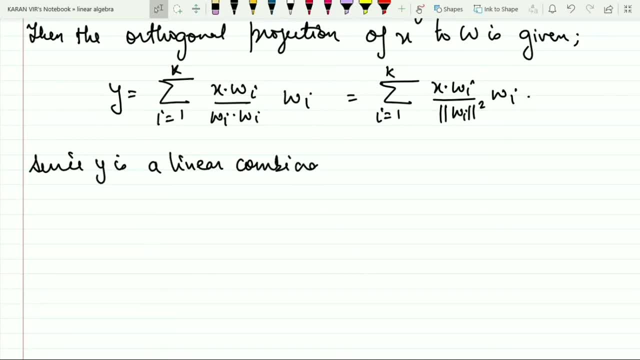 say y is a linear combination, linear combination of w1, w2, up till so on to wk, right. so it belongs to w right. so now, if you calculate x minus y dot with wj, so what does it comes out to be? so it comes out to be x minus. what is the value of y y summation? i, running from 1 to k, right x dot wi. 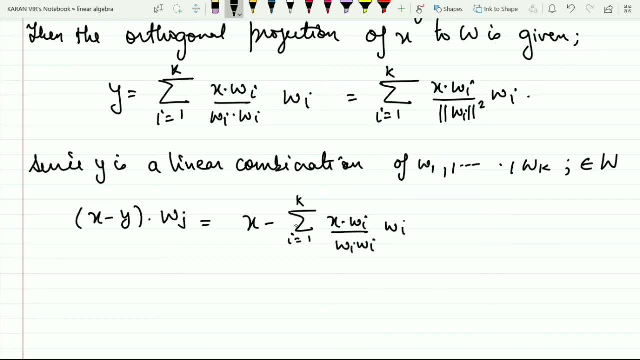 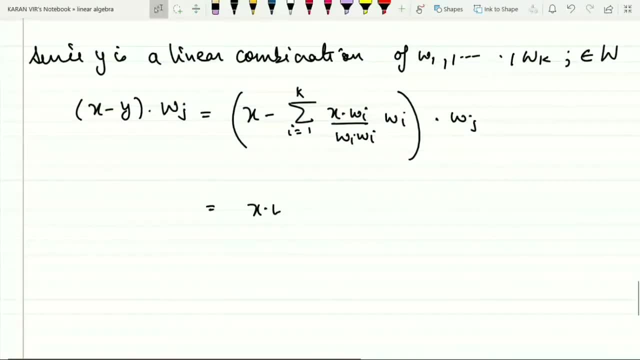 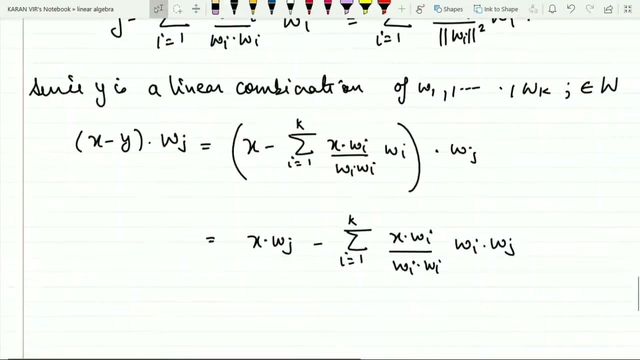 divided by wi dot with wi, multiply with wi and whole dot with wj. now just club the terms. so this is x dot, wj, minus summation. i running from 1 to k: x dot, wi divided by wi dot with wi and wi dot with wj, and in the beginning we have considered wi is to be the orthogonal basis, right? so if they are, 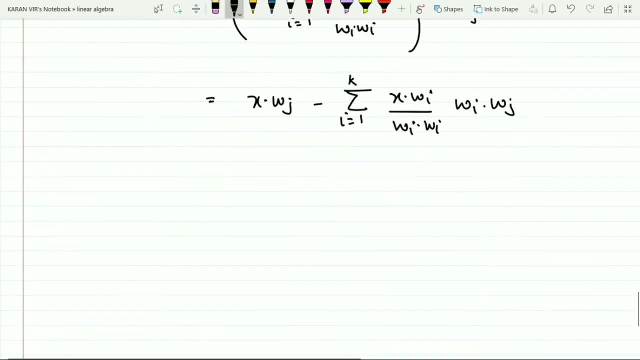 the orthogonal basis. so you will apply the property of orthogonal basis. and you will apply the property of orthogonal basis. so, since they are the orthogonal, so whenever my i is equal to j, so in that case it will be as it is. in all other cases it will come out to be zero. so since they, 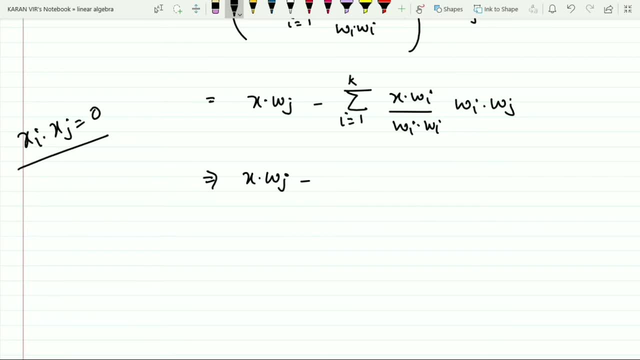 are orthogonal. so it means xi dot with xj they are. that is equal to zero. fine, so whenever my i will equal to bj, so whenever my i will be equal to j, only that vector will be left. so this will be x dot, wj divided by wj dot with wj into wj dot with wj. in all other cases it will come out to be: 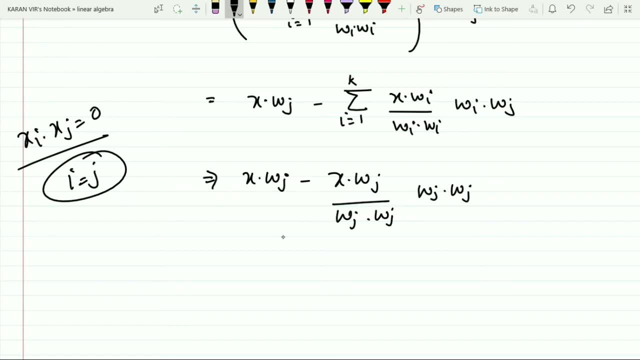 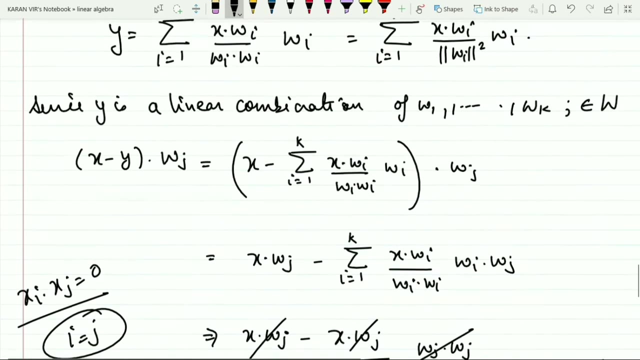 zero in rest of the cases. fine with this. and now just you can see: so this will get cancelled out and these terms will also get cancelled out and finally, you are left with zero, right? so for all j, this is proof for all j that is coming from 1 till k. fine with this, so you have proved that. 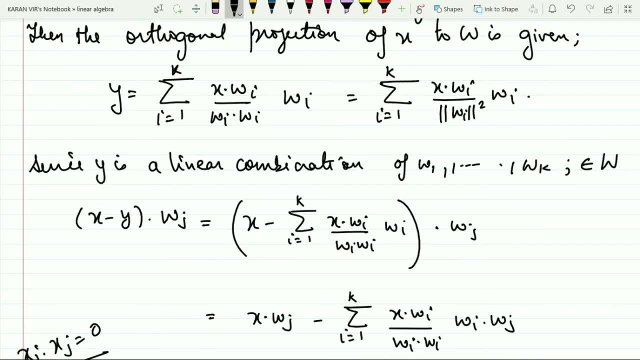 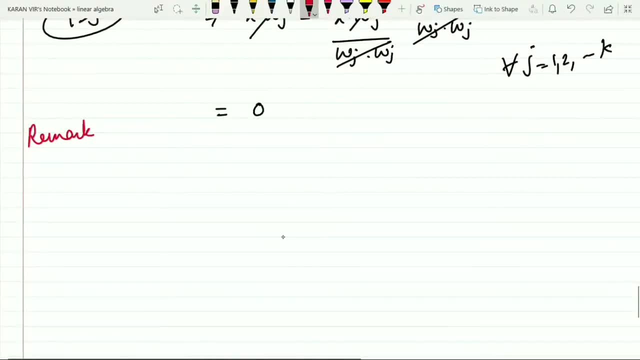 my x minus y dot with wj, that is equal to zero. now what if so? the one one remark before we conclude. when my u1 u2 up till uk, they forms o and b. so if they forms an, o and b? so in that case, what do we have? so y will come out to be equal to summation, because in that case the norm will. 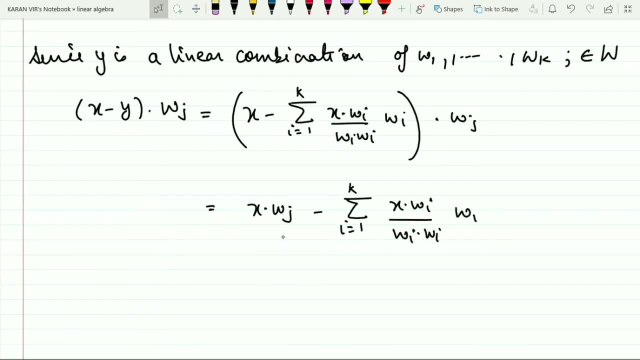 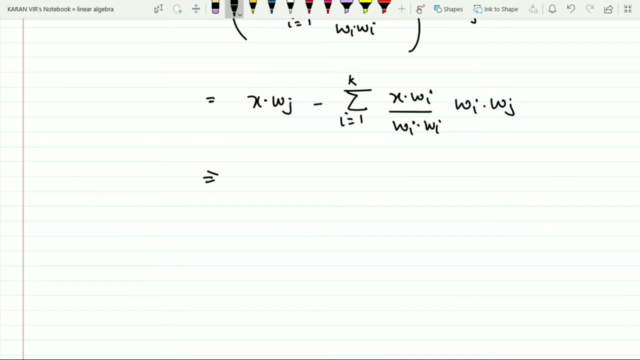 divide by wi dot with wi and wi dot with wj. and in the beginning we have considered wi is to be the orthogonal basis, right? so if they are the orthogonal basis, so you will apply the property of orthogonal basis. so since they are the orthogonal, so whenever my i is equal to j, 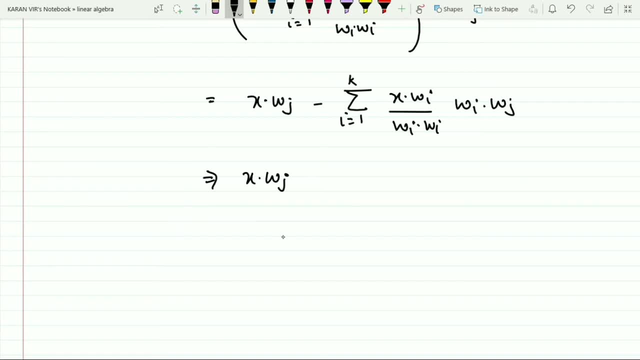 so in that case it will be as it is, and all other cases it will come out to be zero. so since they are orthogonal, so it means xi dot with xj there, that is equal to zero. fine, so whenever my i will equal to be j. so whenever my i will be equal to j, only that vector will be left. so this will be x. 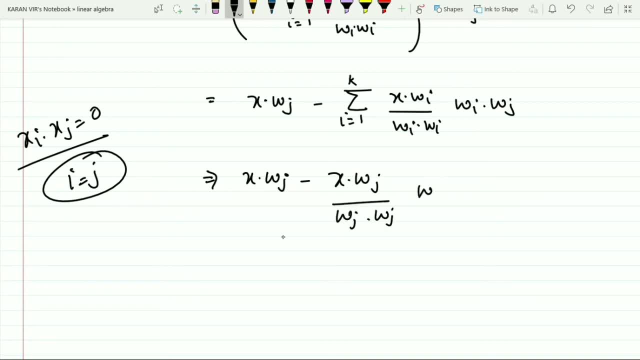 dot, wj divided by wj dot with wj into wj, dot with wj. in all other cases it will come out to be zero in rest of the cases. fine with this. and now just you can see. so this will get cancelled out and these terms. 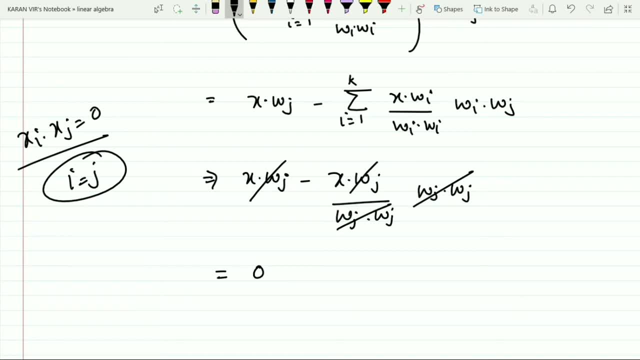 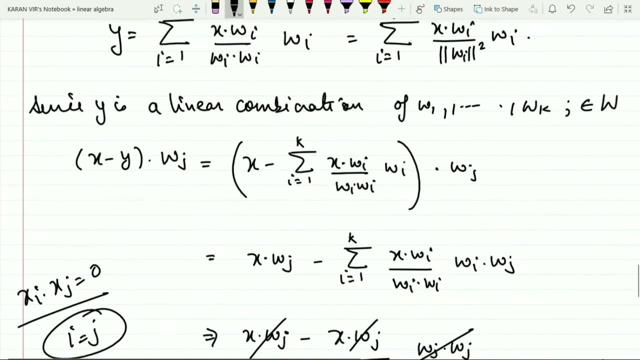 will also get cancelled out and finally you are left with zero right. so for all j, this is proof for all j that is coming from 1 to k. fine with this. so you have proved that my x minus y dot with wj, that is equal to zero. 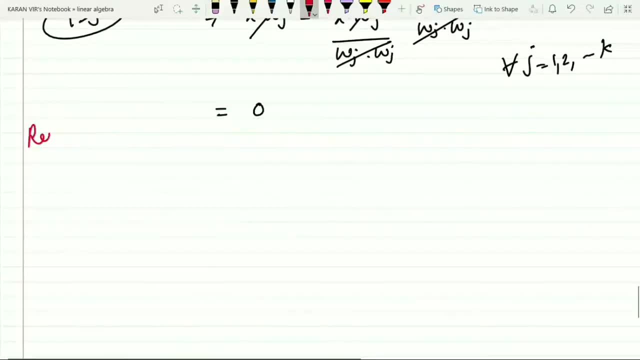 now what if? so the one one remark before we conclude this. so what if, when my u1 u2 up till uk, they forms o and b? so if they forms an, o and b? so in that case, what do we have? so y will come out to be equal to summation, because in that case the norm will come out to be one. so i, running from, 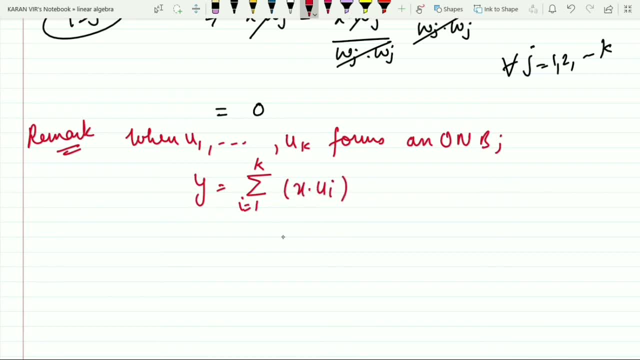 1 to k right x dot u i and multiply with u i. fine, now why this thing is true? because we know that u i dot with u i is equals to 1 for all i right for i running from 1 to k. so that is why this. 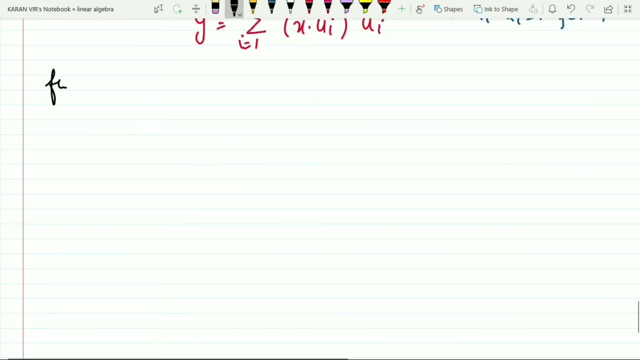 thing is true. now let's see. now let's see, for k equals to 1, what are what the above formula becomes. so it will be equal to x dot w right, w1 divided by w1 dot. w1 multiply with w1. and if my w1 is 1, 1, 1, as i have considered above, and my x vector is x y, z, so in that case you can see that. 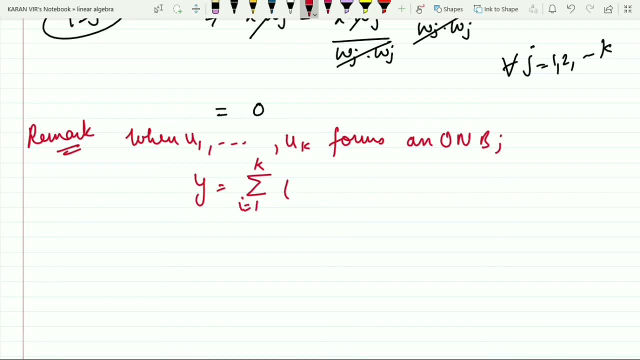 come out to be 1. so i, running from 1 to k, right x, dot, ui and multiply with ui. fine, now why this thing is true? because we know that. because ui, dot with ui, is equals to 1 for all, i right for y, running from 1 to k. so that is why this thing is true. now let's see. now let's see for k equals. 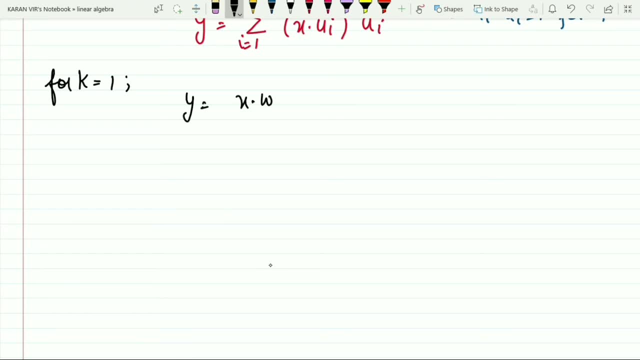 to 1, what are what the above formula becomes. so it will be equal to x dot w right w1 divide by w1 dot, w1 multiply with w1. and if my w1 is 1, 1, 1, as i have considered above, and my x vector is x, y, z, 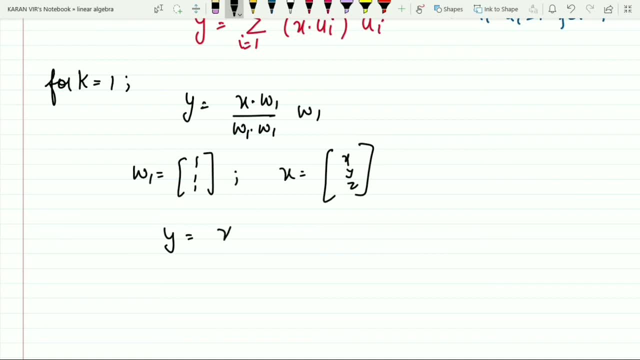 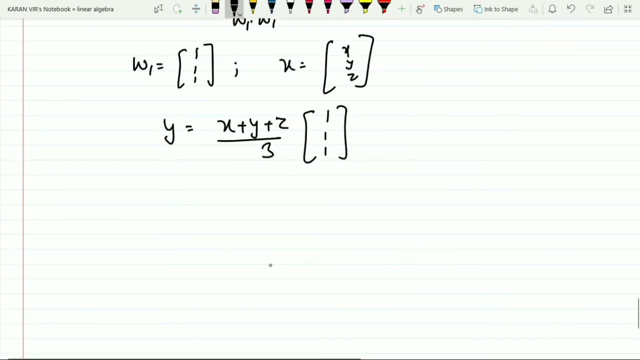 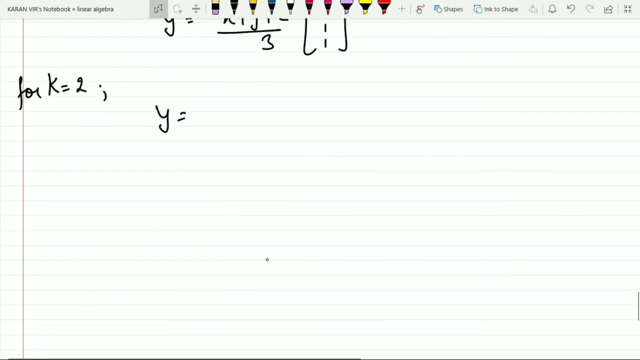 so in that case you can see that my y vector will come out to be equal to x plus y plus z. divide by 3. multiply with 1. 1 and 1 for k equals to 2. so what does the above formula become? so the above formula becomes: y equals to x. dot w1. divide by w1. 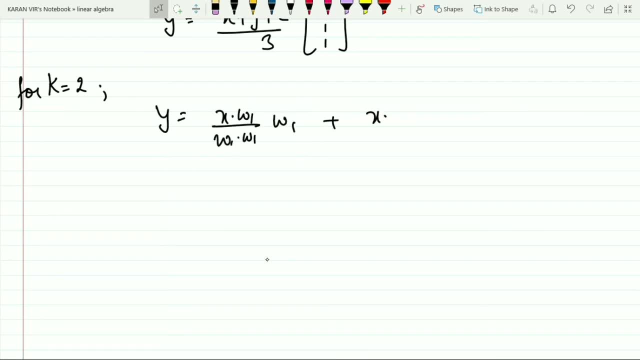 dot w1. multiply with w1 plus x dot w2. divide by w2. dot with w2. multiply with w2 right. and in the similar way you can consider w1 to be 1 minus 1 and 0. fine, w2 that is equals to 1: 1. 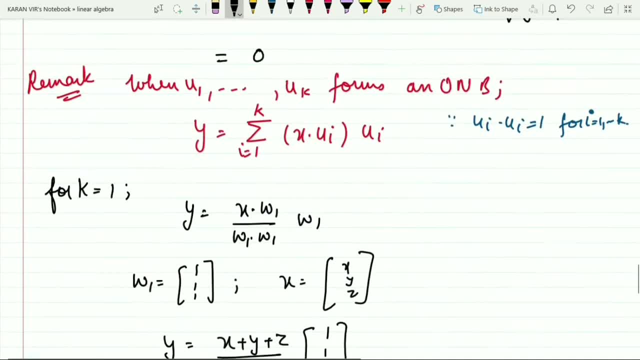 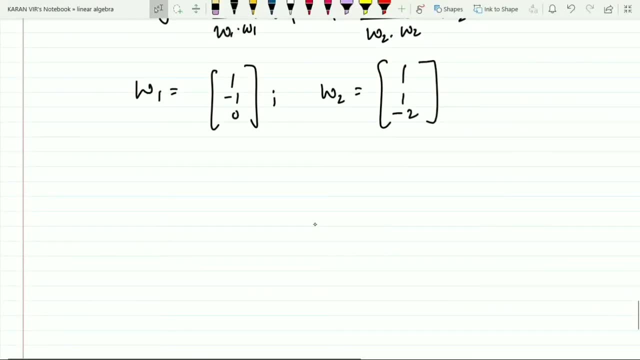 and minus 2. so, students, you should recall that these wis, they should be orthogonal basis and you can check that this is an orthogonal basis, right? w1 dot with w2 is equals to 0. so since, since w1, w2 are orthogonal, so they are orthogonal, so you can calculate the projection. 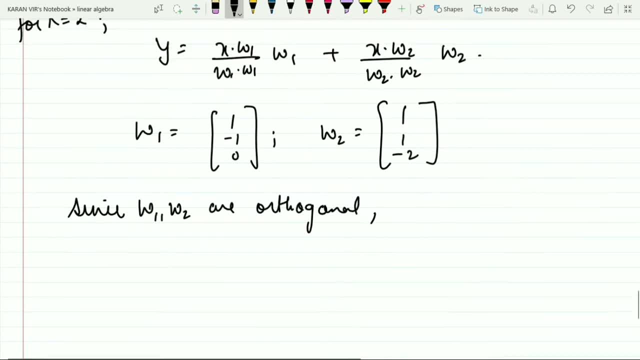 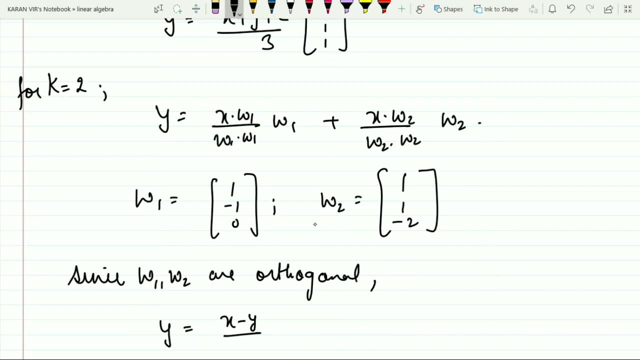 right and we have written the formula and above right. so y comes out to be x dot w1. so in that case it will be x minus y. right divide by the norm of w1. so the norm of w1 square, that is a 2 multiply with w1, that is 1 minus 1 and 0. fine, x dot with w2 will come out to be x plus y. 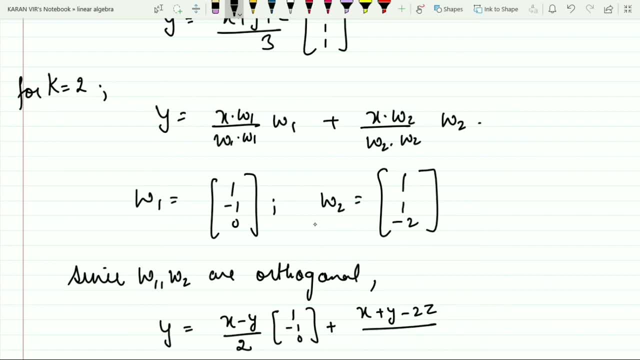 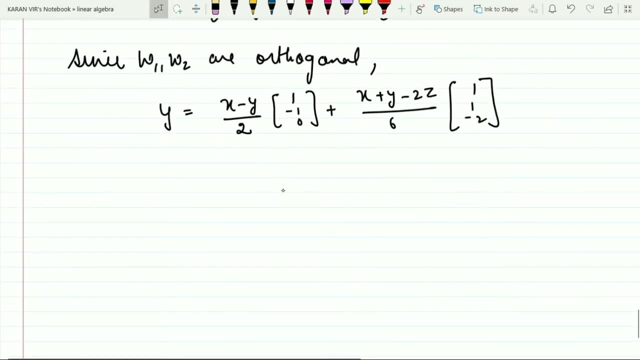 minus 2z. divide by the norm square of w2, that comes out to be 6, right, and multiply with 1 minus 1, so 1, 1 and minus 2, and finally, if you solve these equations, so finally, what will be the answer? so, 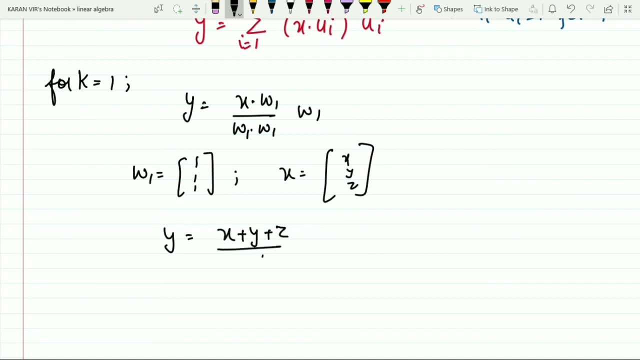 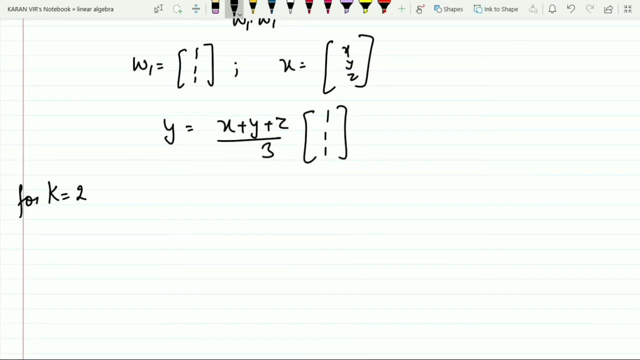 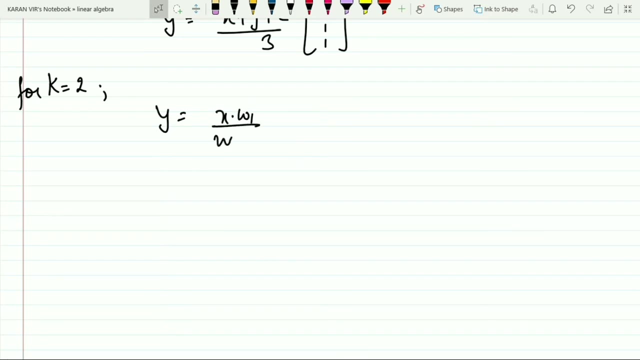 my y vector will come out to be equal to x plus y plus z. divide by 3. multiply with 1. 1 and 1 for k equals to 2. so what does the above formula become? so the above formula becomes: y equals to x. dot. w1. divide by w1 dot. w1 multiply with w1 plus x. dot. w2. divide by w2 dot with w2. multiply with. 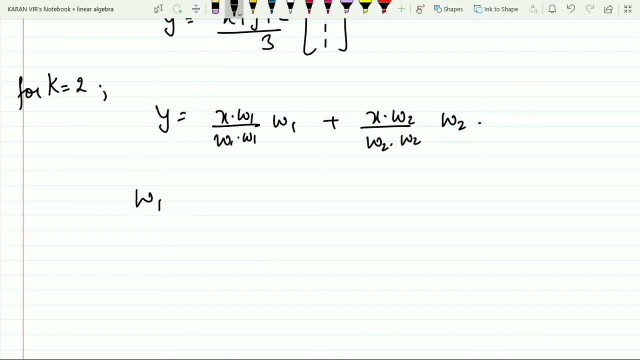 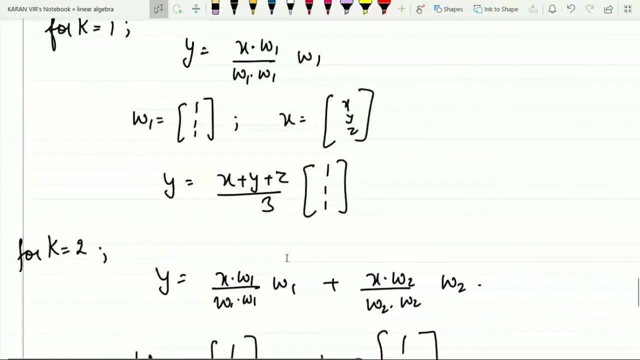 w2 right, and in the similar way you can consider w1 to be 1 minus 1 and 0. fine, w2 that is equals to 1, 1 and minus 2. so, students, you should recall that these w i's, they should be orthogonal basis and you can check that this is an orthogonal basis. 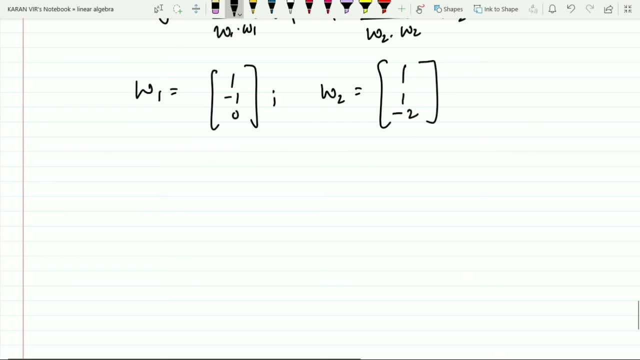 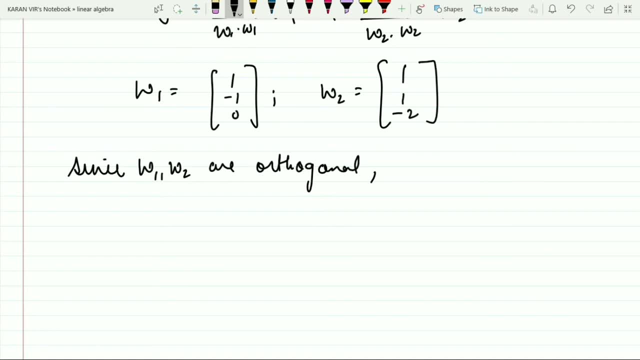 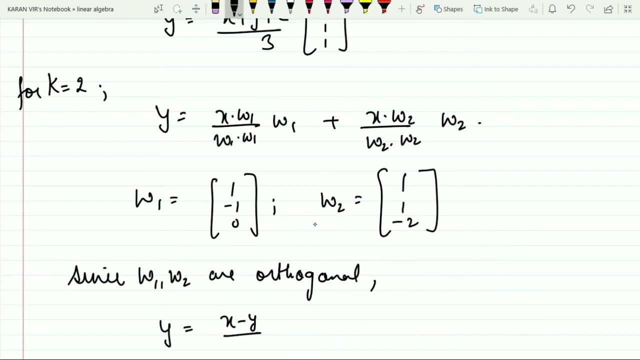 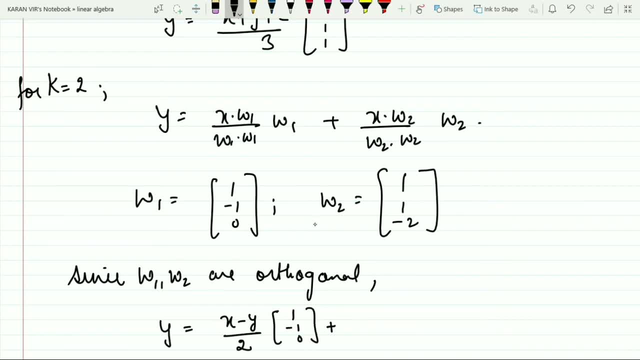 multiply with w1, that is 1 minus 1 and 0. fine, x dot with w2 will come out to be x plus y minus 2. z divided by the norm square of w2, that comes out to be 6, right, and multiply with 1 minus 1. so 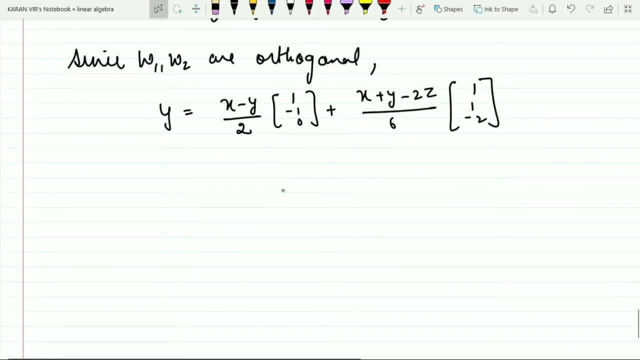 1, 1 and minus 2 and finally, if you solve these equations, so finally, what will be the answer? so the answer will be 1 by 3 common, so 2x minus y minus z, minus x plus 2y minus z, and the final will be minus x minus y plus 2z. so that will be the final answer. 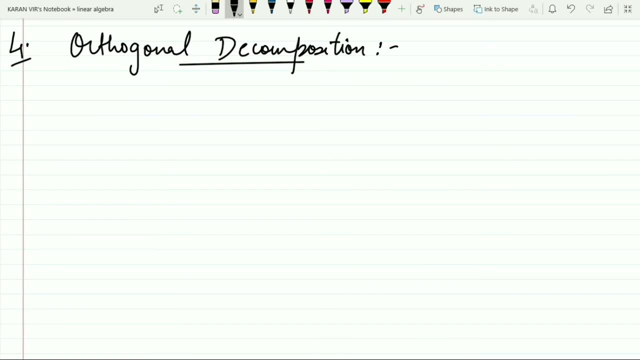 if you calculate the above things. so the fourth topic for the day is orthogonal decomposition. right again for this. so very simple topic actually. so let w be a linear subspace, linear subspace of Rn, and again, let x be any vector that is coming from Rn, right? 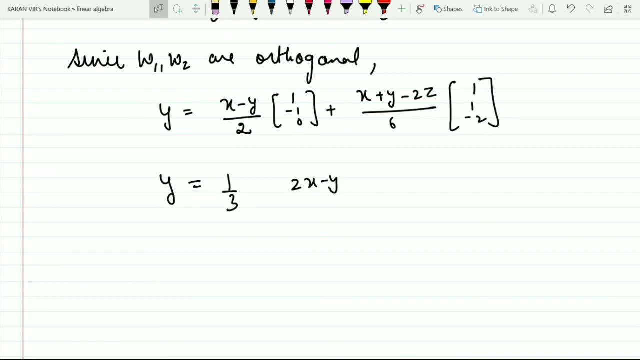 the answer will be 1 by 3 common, so 2x minus y minus z minus x plus 2y minus z, and the final will be minus x minus y plus 2z. so that will be the final answer if you calculate the above things. 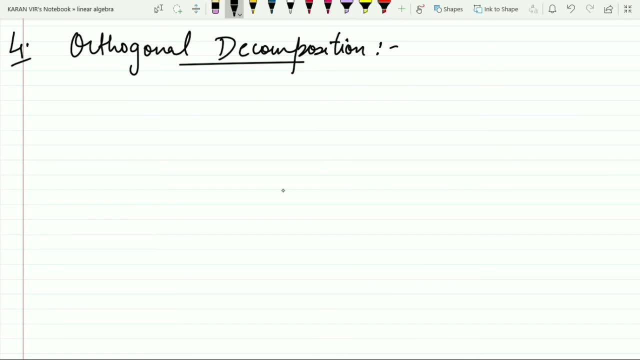 so the fourth topic for the day is orthogonal decomposition. right again for this. so very simple topic actually. so let w be a linear subspace, linear subspace. so and again, let x be any vector that is coming from rn, right, and you, as we consider y to be the. 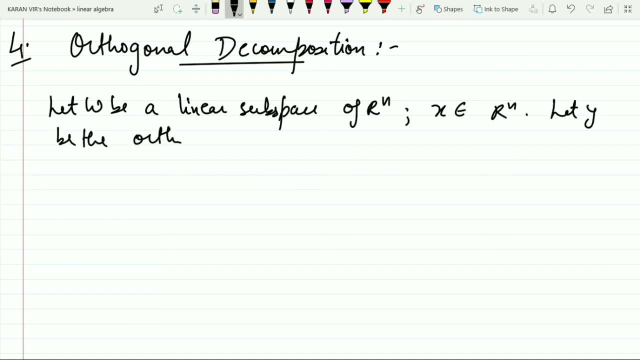 so y be the orthogonal projection, orthogonal projection of this vector x right to the subspace w, then the vector, then the vector y and z. what was my z? that is x minus y, so they satisfy a property. so they satisfy a property, and then the vector y and z, which is the vector y and z. 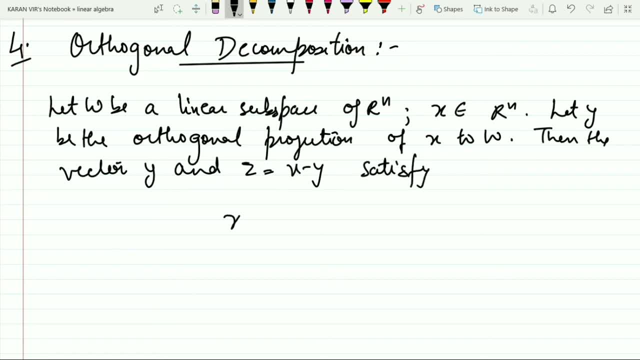 satisfy, that is, you can say that x is equals to y plus z, where my y is coming from w and z is coming from w, perpendicular. So you have, you know, decomposed this vector x into two parts, where the first part is coming from w and the second part is coming from w, perpendicular, right. So such an? 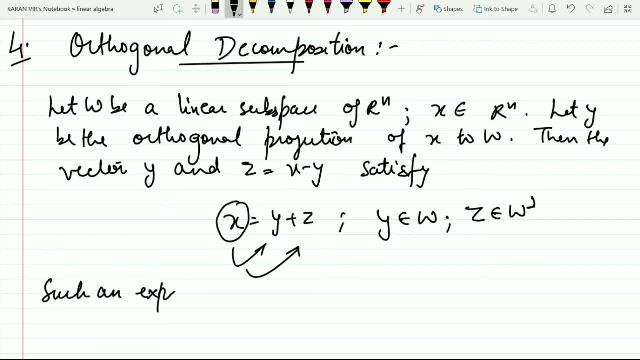 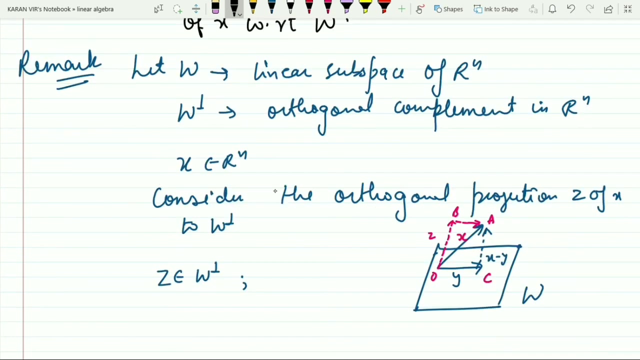 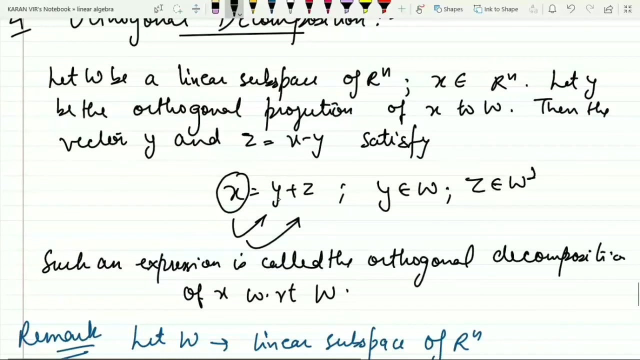 expression. such an expression is called the orthogonal decomposition, orthogonal decomposition of x with respect to the subspace w. Fine, with this. So before we conclude this lecture, let me add a remark. So the previous formulas were: what is the orthogonal projection Right of this vector to the subspace w? What, if I get find the orthogonal projection of this? 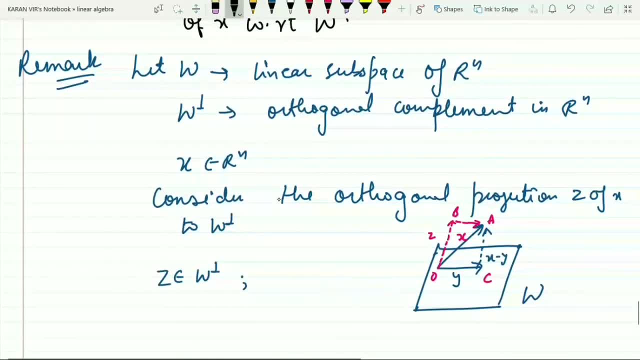 x to the subspace that is a perpendicular subspace, that is, w perpendicular. For this, let me consider w to be a linear subspace of Rn and w perpendicular, that is, orthogonal complement of in Rn right, and x be any vector that is coming from Rn. Now you consider the. 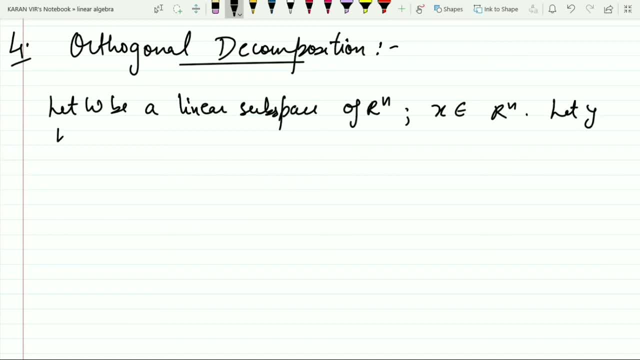 and you, as we consider y to be the, so y be the orthogonal projection, orthogonal projection of this vector x right to the subspace. w, then the vector, then the vector y and z. what was my z? that is x minus y. so this satisfy a property, so this satisfy that is. 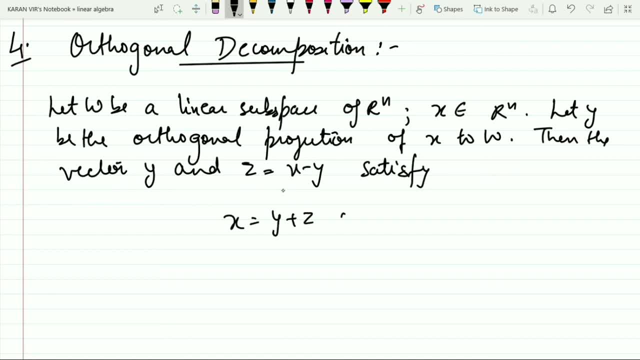 you can say that x is equals to y plus z, where my y is coming from w and z is coming from w- perpendicular. so you have, you know, decomposed this vector x into two parts, where the first part is coming from w and the second part is coming from w- perpendicular, right. so such 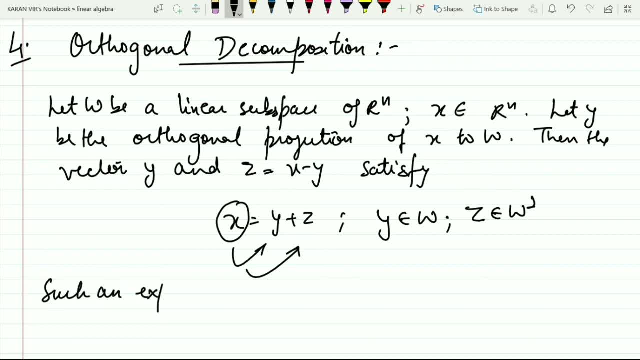 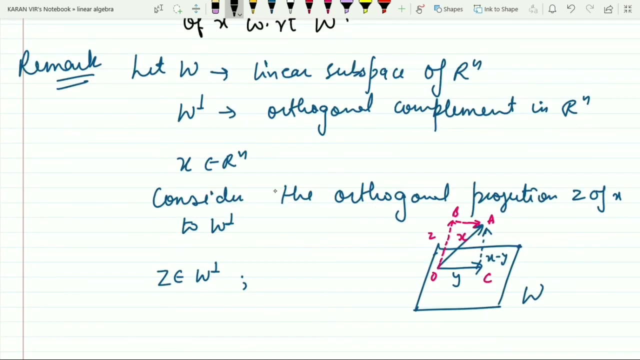 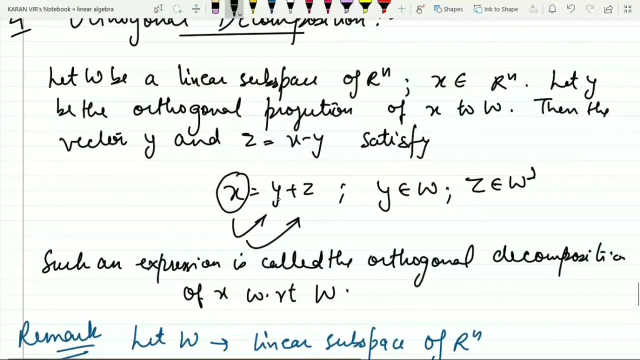 an expression. such an expression. such an expression is called the orthogonal decomposition. orthogonal decomposition of x with respect to the subspace. w fine, with this. so before we conclude this lecture, let me add a remark. so the previous form will: what is the orthogonal projection right of this vector to the subspace? w? what if i get particles of w? right, i get. so, basically, when we apply this條, we can said: Kontakt Zy arguments right, because b and z are in the area first rank of 0 and you can say that we have been operation when we make the choose the first rank of n and only z in the area pieces after z replaced with z and the сразу. 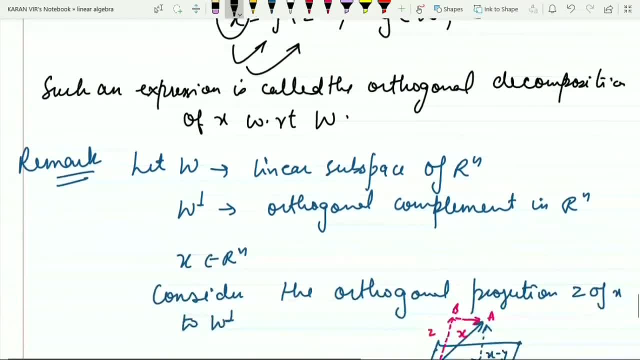 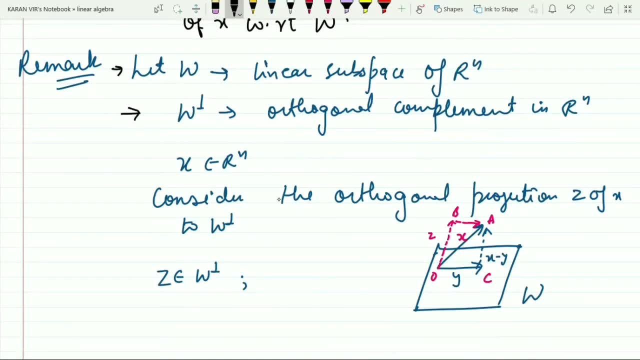 the orthogonal projection of this x to the subspace that is, a perpendicular subspace, that is, w perpendicular. for this, let me consider w to be a linear subspace of rn and w perpendicular, that is, orthogonal complement of in rn right, and x be any vector that is coming from rn. 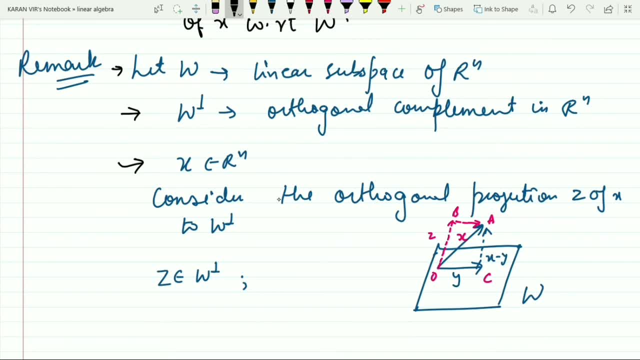 now you consider the orthogonal projection z of x to the w perpendicular subspace. so clearly you can see. so this is my vector is x, right, and this is my vector y. so this will be x minus y from the triangle slope. now just complete the triangle which i have marked with the pink color right. so 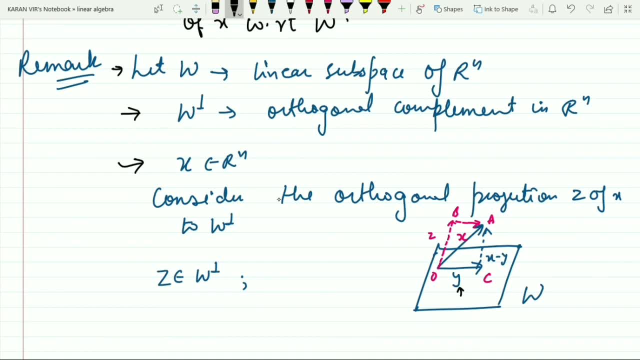 this will be z, so this will be ba. so what will be my ba? that will be x minus right. so x minus z. fine with this. so if i say my z is coming from w perpendicular, so what is my x minus y? that is my z. so z belongs to w perpendicular. yes, this thing is true. so my x minus z. so that is a vector which. 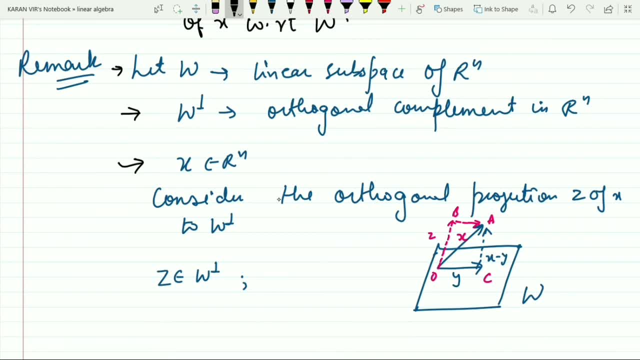 orthogonal projection z of x to the w perpendicular subspace. So clearly you can see. so this is my vector x, right, and this is my vector y. so this will be x minus y from the triangle's law. now just complete the triangle which i have marked with the pink color right. so this will be z. so this will be. 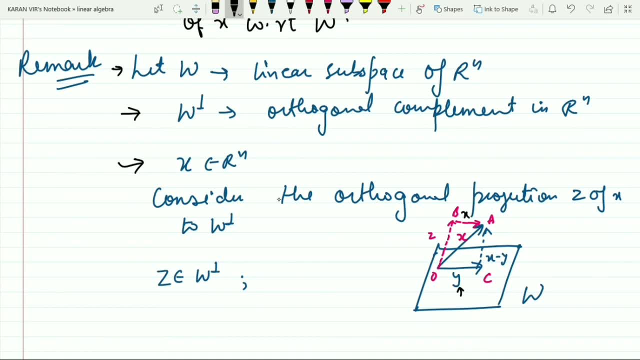 b a. so what will be my b a? that will be x minus right. so x minus z. fine with this. so if i say my z is coming from w perpendicular, so what is my x minus y? that is my z. so z belongs to w perpendicular. yes, this thing is true. so my x minus z. so that is a vector which is, you know, parallel. 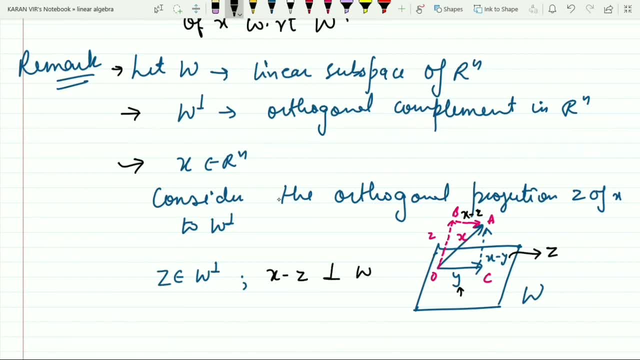 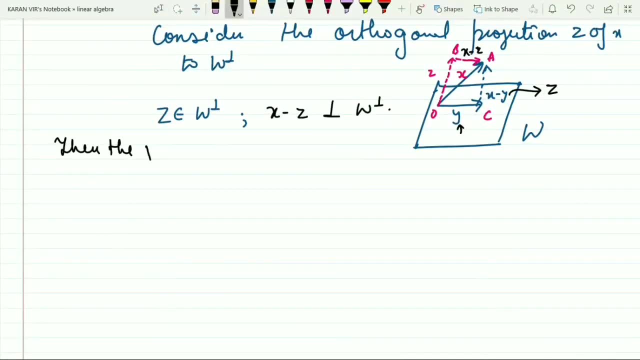 to y. so can i say this: x minus z is perpendicular to this subspace, w perpendicular right. so the same intuition is clear. so that is then the vector y. so what is my vector y? that is x minus z. so this agrees with the orthogonal projection. this agrees with the orthogonal projection of x to w. so can i? 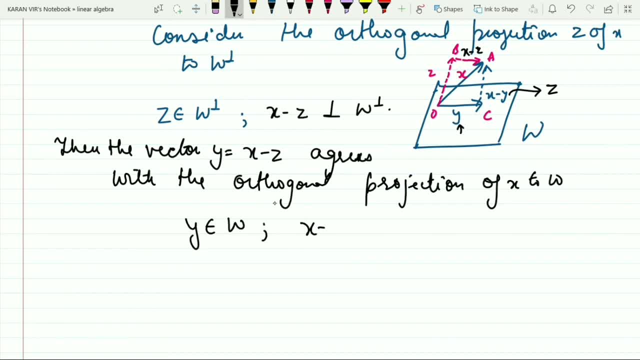 say that my y belongs to w right and x minus y is perpendicular to w. fine with this. so therefore, if w1 up till so on to wk, they are the set of orthogonal bases of w. so what will be the formula? the formula will be: z equals to x minus y, and we know that. what is? 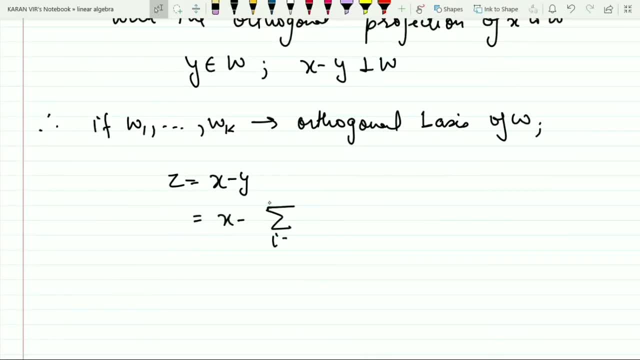 my y, y is nothing but the summation right. i running from 1 to k: x dot. wi divide by wi. dot with wi, multiply with wi. so this gives me the orthogonal projection. so this gives me the orthogonal projection of x to the perpendicular subspace that is a w. 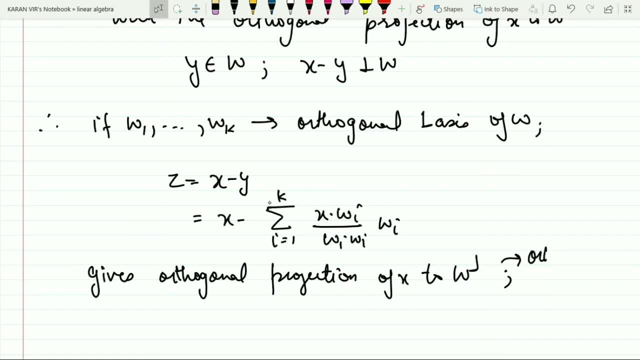 perp, right? so what is the w perp? that is the orthogonal complement of w. so i hope this formula is clear to you now. so what is the formula? final, final formula is this one. so if you want to, the orthogonal projection of x to the perpendicular subspace, and what if you want to calculate? 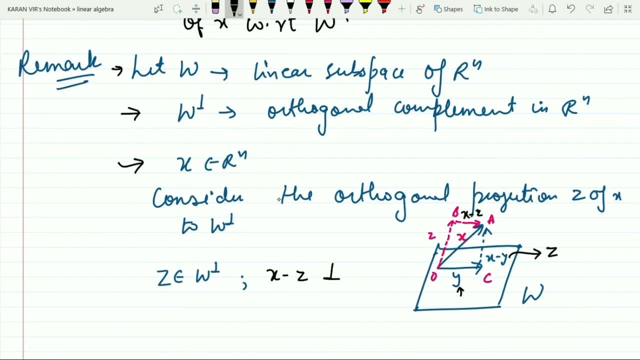 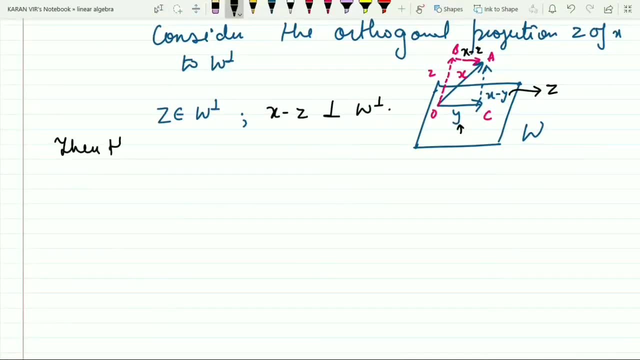 is, you know, parallel to y. so can i say this: x minus z is perpendicular to this subspace, w perpendicular right. so the same intuition is clear. so that is then the vector y. so what is my vector y? that is x minus z. so this agrees with the orthogonal projection. this agrees with the. 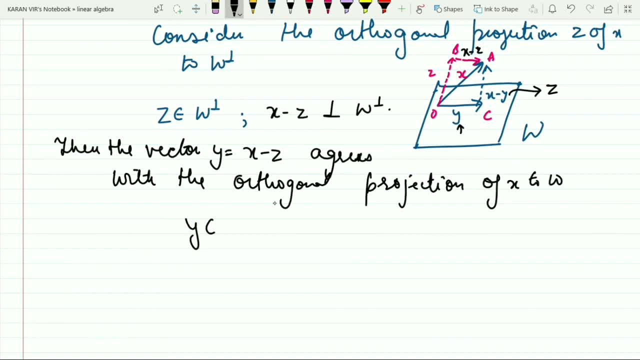 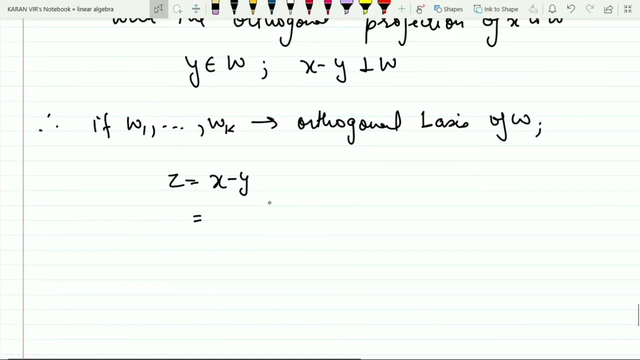 orthogonal projection of x to w. so can i say that my y belongs to w right and x minus y is perpendicular to w. fine with this. so therefore, if w1 up till, so on to wk, they are the set of orthogonal bases of w. so what will be the formula? the formula will be: z equals to x minus y, and we know that. what is? 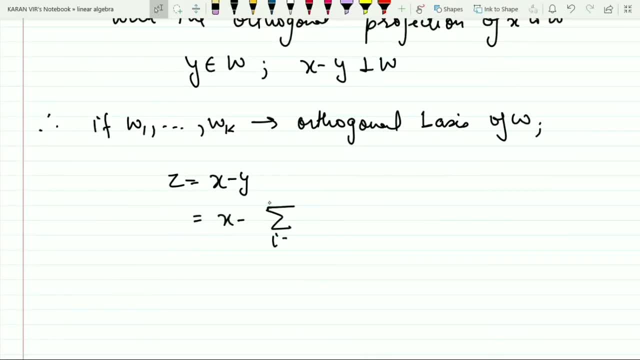 my y, y is nothing but the summation, right. i, running from 1 to k: x dot. wi divide by wi, dot with wi multiply with wi. so this gives me the orthogonal projection. so this gives me the orthogonal projection of x to the perpendicular subspace. that is a w bar, right? so what is the w bar? that is the. 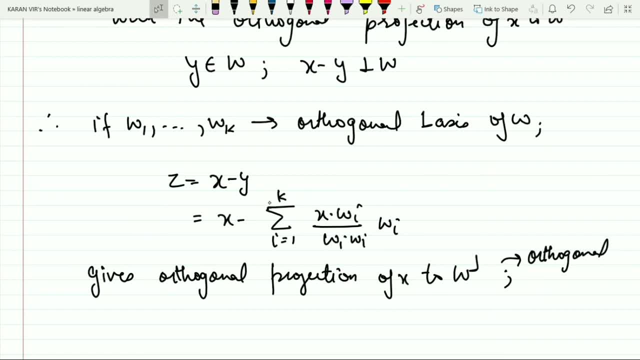 orthogonal complement of w. so i hope this formula is clear to you now. so what is the formula? final, final formula is this one. so if you want to calculate the orthogonal projection of, if you want to calculate the orthogonal projection of x to the perpendicular subspace, and what if? 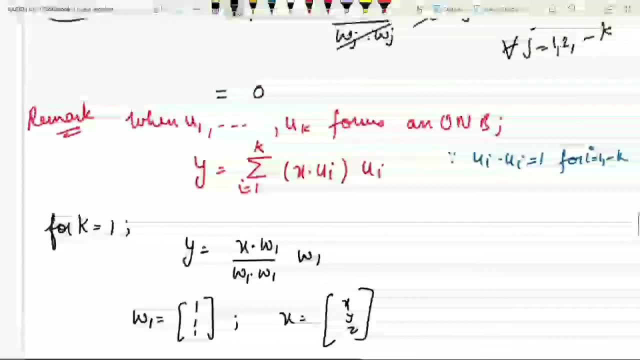 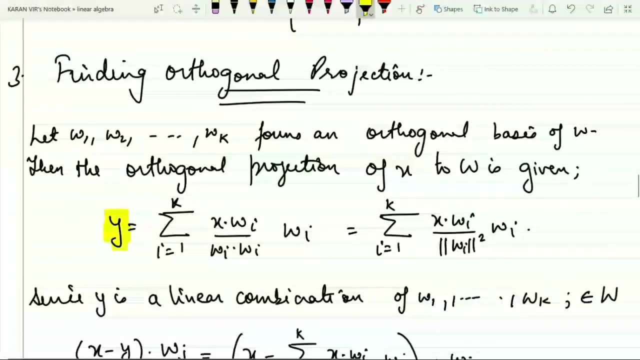 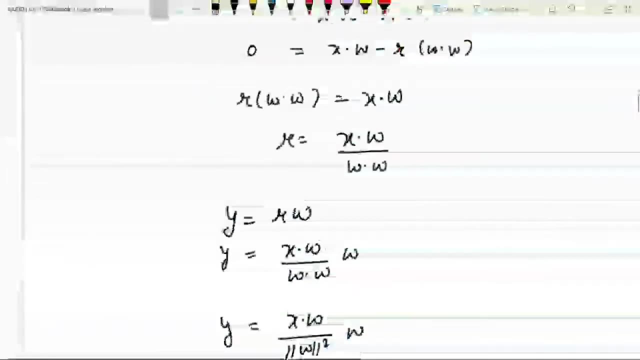 want to calculate normal projection of the vector x right. so for that you know what is the formula. the formula is given here, so let me mark it again. so that is, y equals to summation this right x dot wi divided by the norm of wi square into wi. so i hope all these four topics which i have discussed 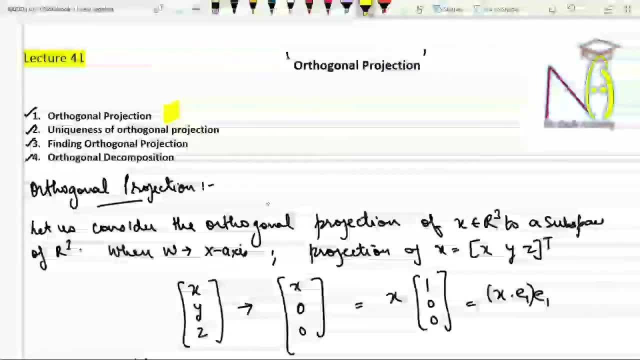 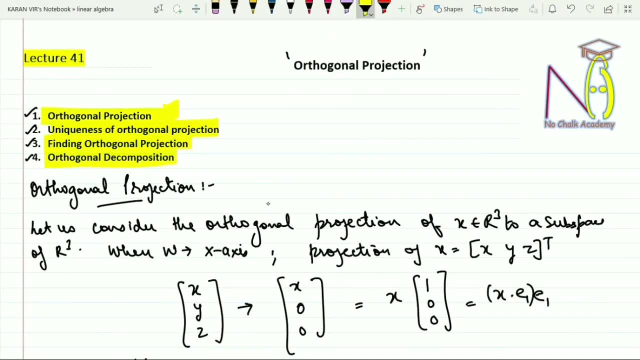 in this video lecture, that is, orthogonal projection, right, and the second one is the uniqueness of orthogonal projection, then the finding, orthogonal projection and orthogonal decomposition. i hope these four topics are clear to you now in the in the upcoming video lectures we will be exploring few more concepts, right, and i hope you have enjoyed this video session for more such videos. 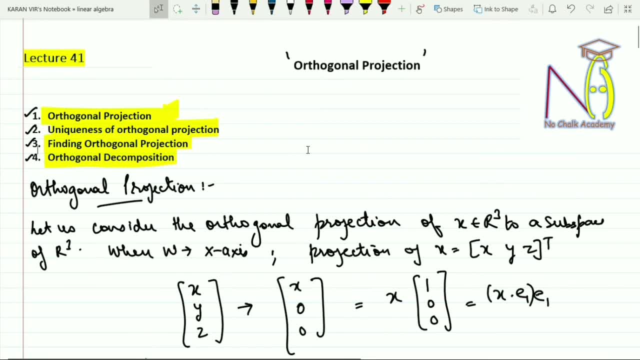 do subscribe to my youtube channel and do not forget to press the bell icon. thank you so much, students. thank you.